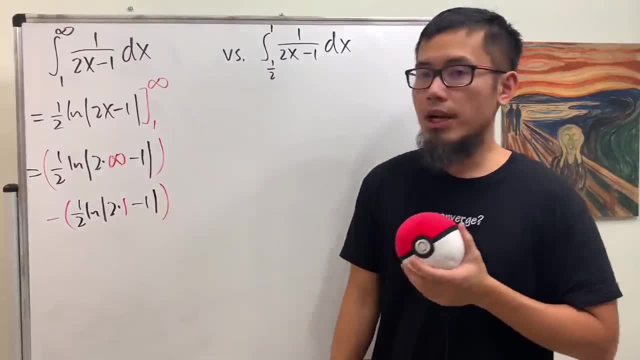 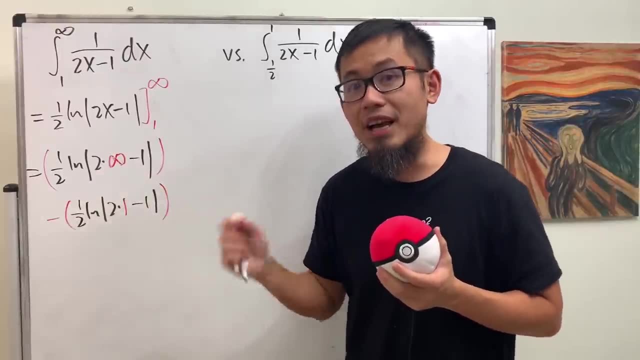 and then minus 1, like so right, So right here. let's see: 2 times infinity is infinity. minus 1 is still infinity. absolute value of infinity is still infinity. ln of infinity is still infinity. minus 1: half is still infinity. yes, just infinity, right here. 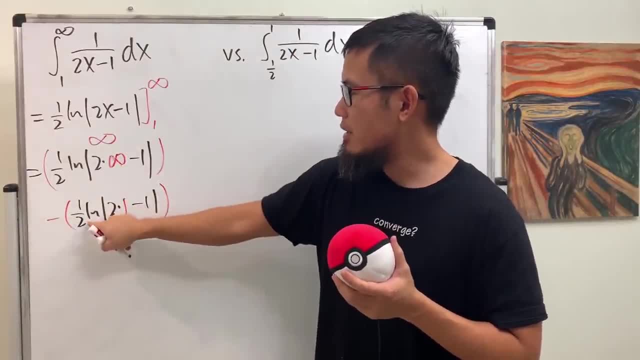 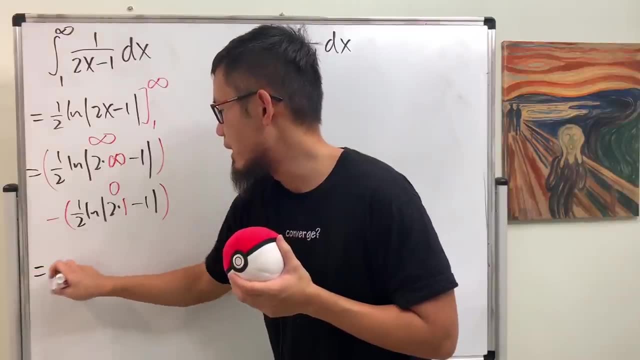 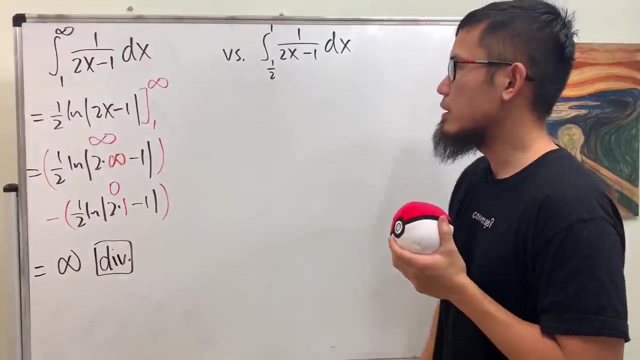 This: 2 times 1, minus 1 is 1, but instead of the ln we get 0 times 1. half is still 0, so this is just infinity minus 0, so we get the whole thing to be infinity. therefore, that integral diverges So, as you can see, that infinite interval. 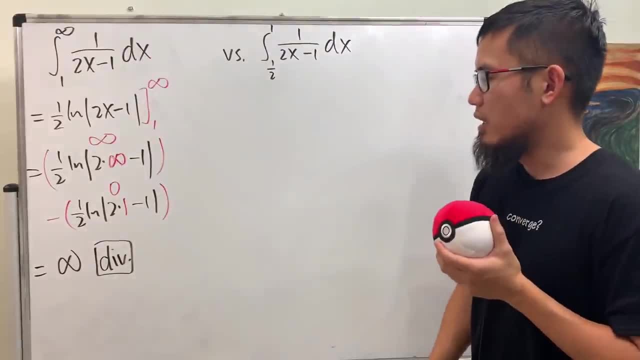 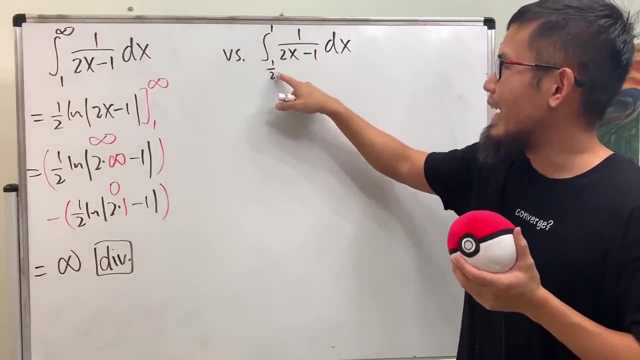 when we go from 1 to infinity. of this, we turn out to get an infinite area. right Now let's see the type of situation of the same function. right here We go from 1 half to 1.. Well, when x is 1, 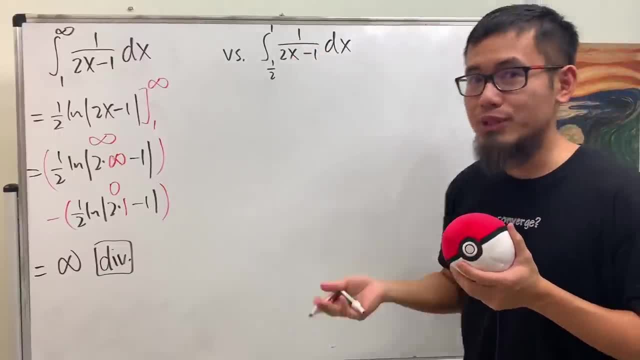 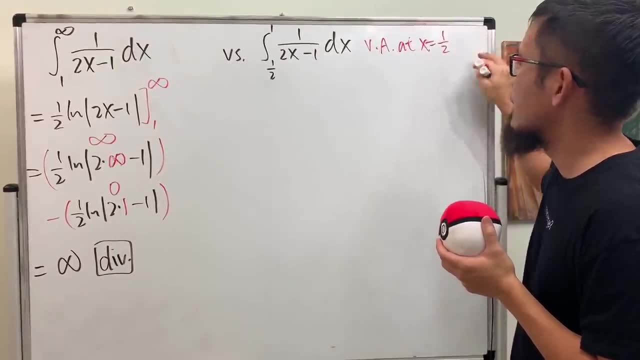 half. when we put it here, we get 1 over 0, we actually have a vertical asymptote. That's why- let me just emphasize this- we have a vertical asymptote at x equal to 1 half. That's why this is a type 2 improper. 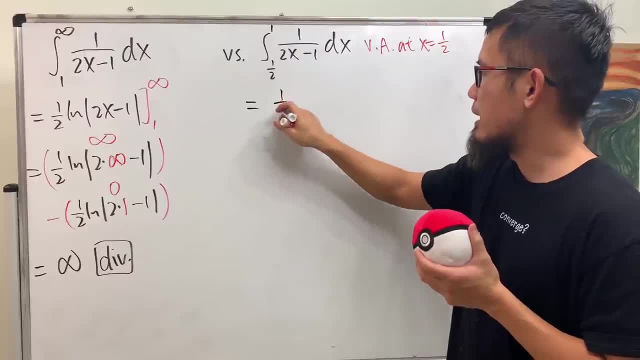 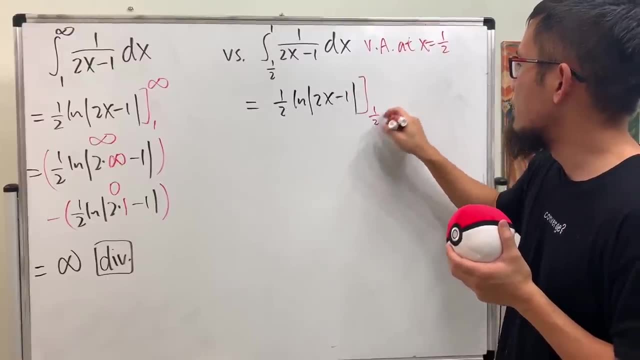 integral. okay, So same integral. just go ahead and put that down like 1 half ln absolute value, 2x minus 1, and then we are going from 1 half to 1, and plug in, plug in. And before we do so, 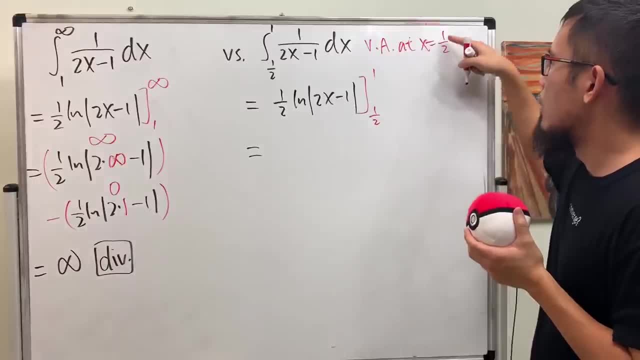 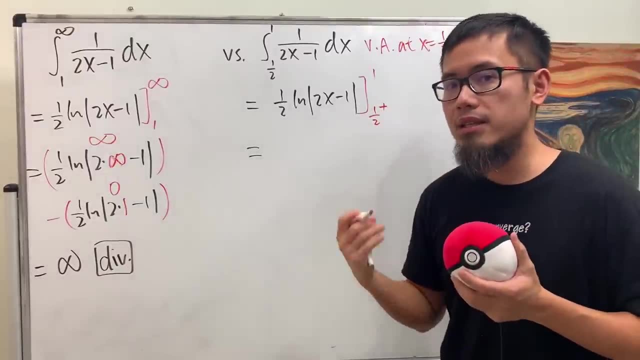 let me just emphasize that, because we do have a vertical, when x is equal to 1 half, this right here is technically 1 half plus. because we have to take the limit, We have to think in terms of limits. All right, plug in 1, we first get 1 half ln. 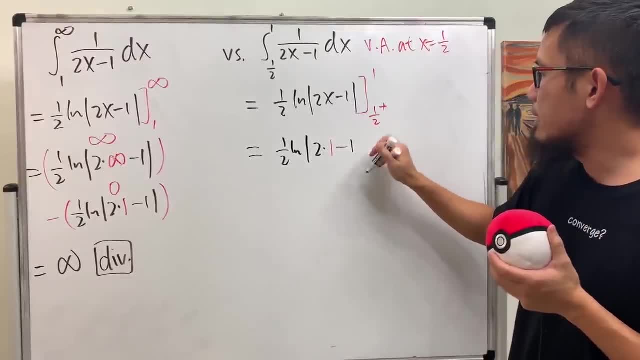 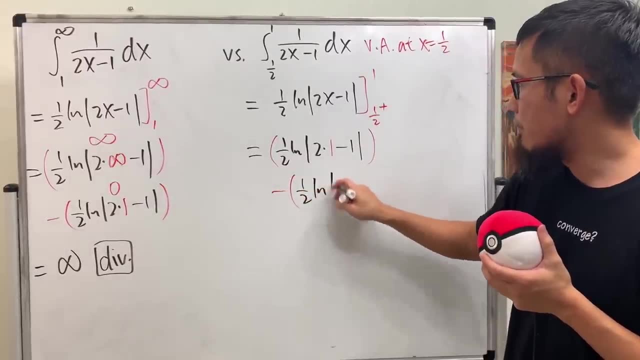 absolute value 2 times 1, and then minus 1 in the absolute value, first part right here and then minus. plug in 1 half plus. so we have this times 1 half plus and then minus 1.. Pretty. 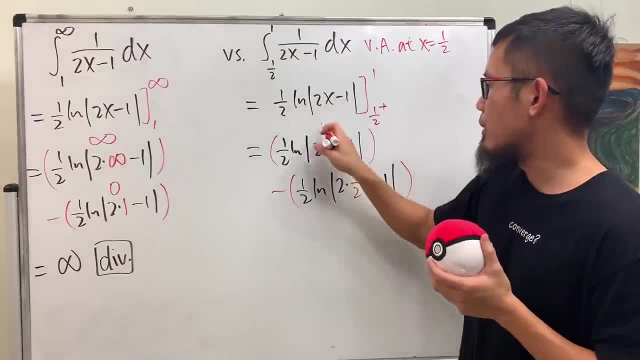 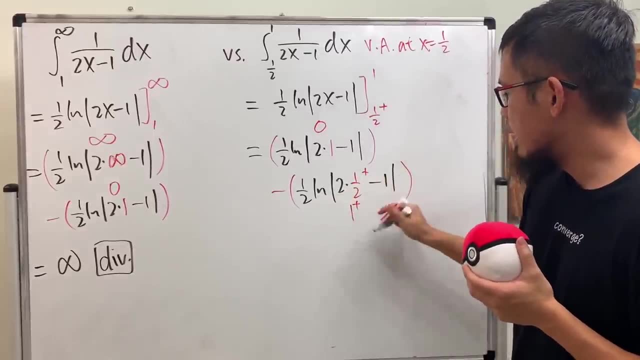 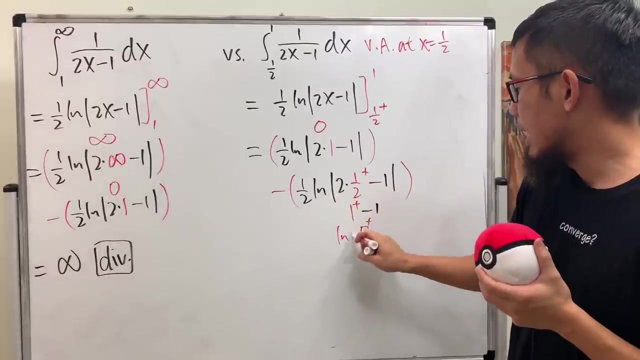 good, All right, for this part we get 0.. For this part, 2 times 1 half plus is 1 plus. So let me just write that down for you guys, and then minus 1, that will be 0 plus And ln absolute value: 0. 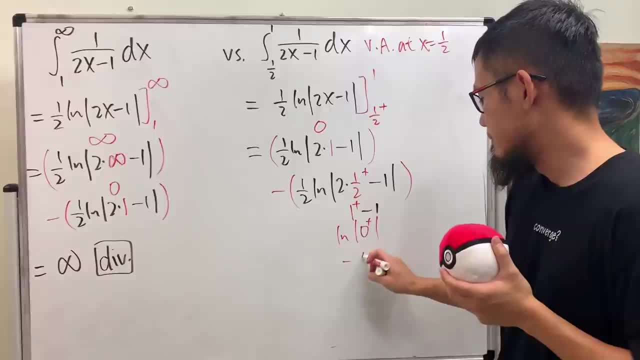 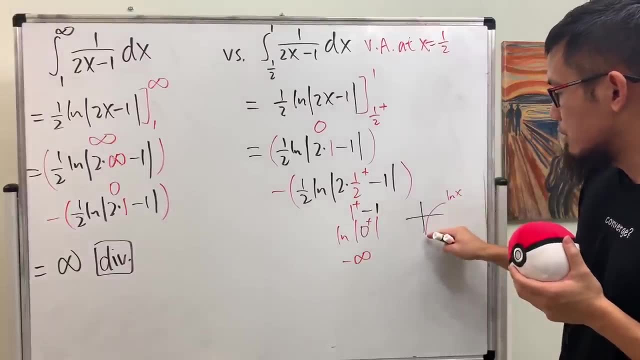 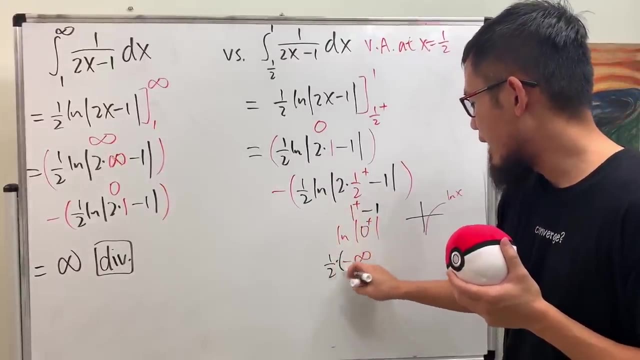 plus, This right here is negative infinity. Remember, when you look at the graph of natural log, if x is approaching 0 from the right-hand side, the graph goes straight down. that's what we get: negative infinity. And then, right here, we just continue. we have the 1 half in front, So 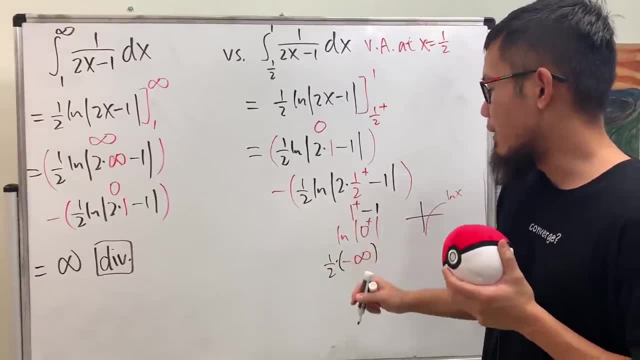 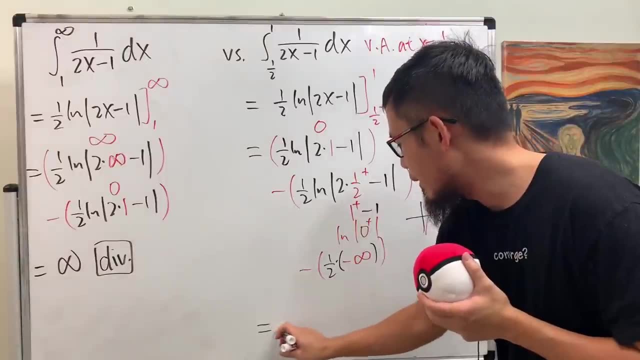 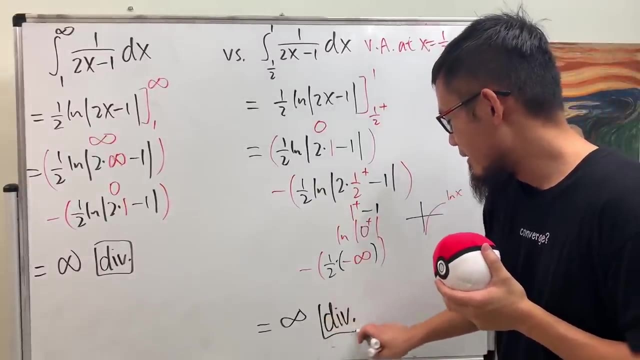 of course that's still negative infinity, but we have this negative in front. So all in all, we get a positive infinity. So 0 plus infinity. we also have infinity right here. Well, kind of weird, Both of them diverge, right, But that might not be the situation. Check out. 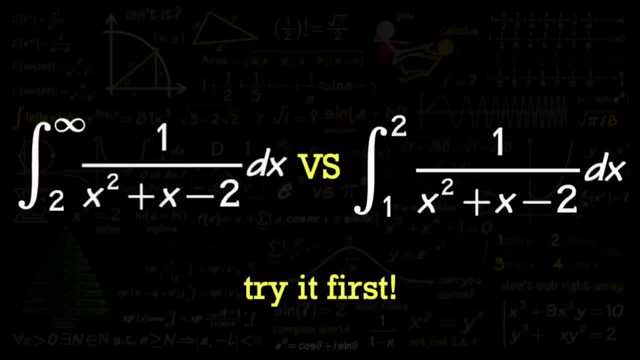 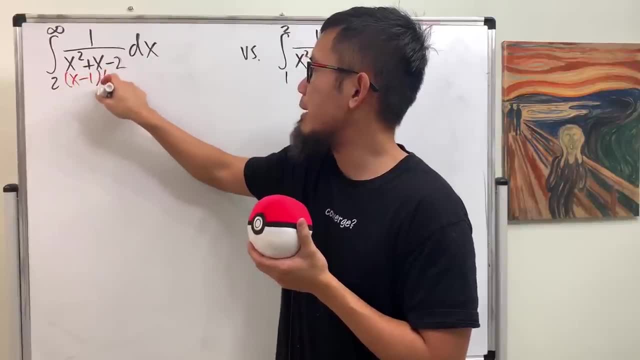 the other questions, This bottom can actually be factored. so to go ahead and do that, we get x minus 1 times x plus 2.. And notice, when x is equal to 1, we will actually get the vertical isotope. 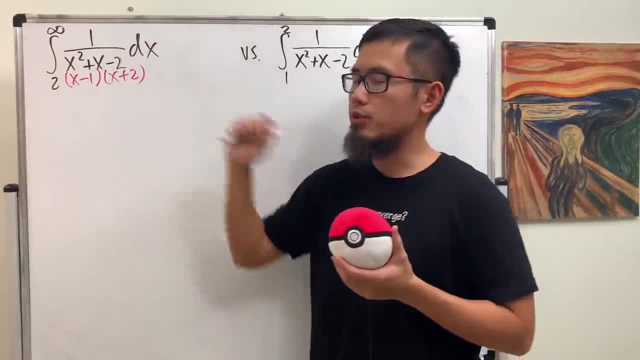 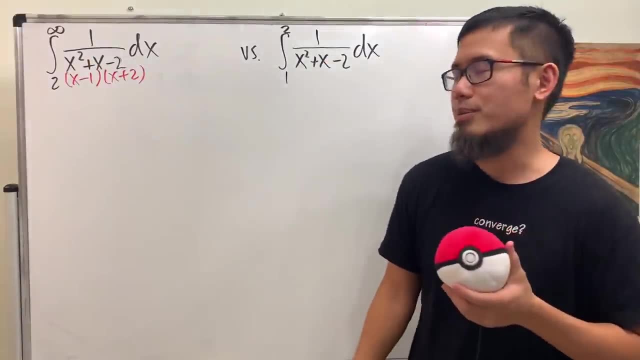 So that's why this right here is the type 2 situation, while this right here is the type 1 situation, because we have infinite interval going from 2 to infinity. But when x is equal to 2, it's not vertical isotope right. 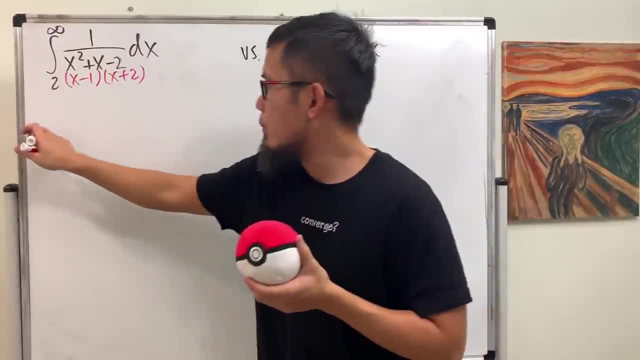 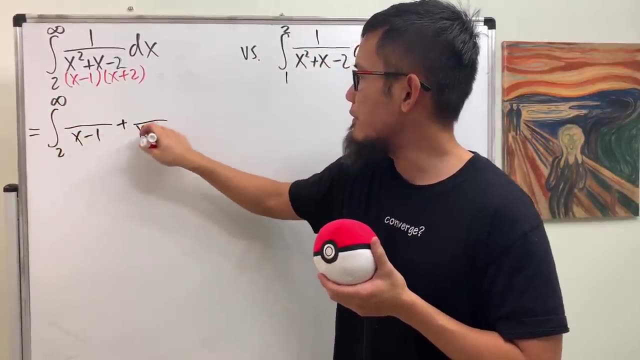 All right. So to integrate this, we'll use partial fractions. Well, let's look at the integral, going from 2 to infinity. The first fraction will have x minus 1 on the bottom, and the second fraction will have x plus 2 on the bottom. And to figure out this number here, well, go back to the. 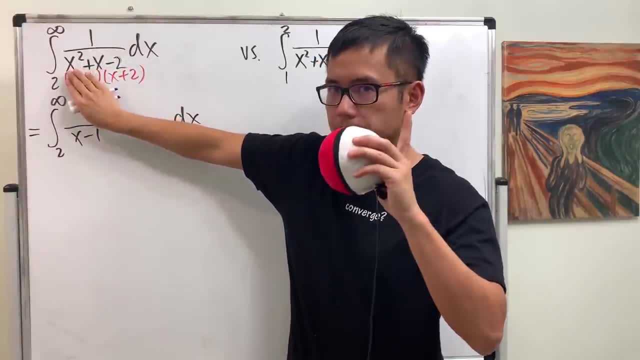 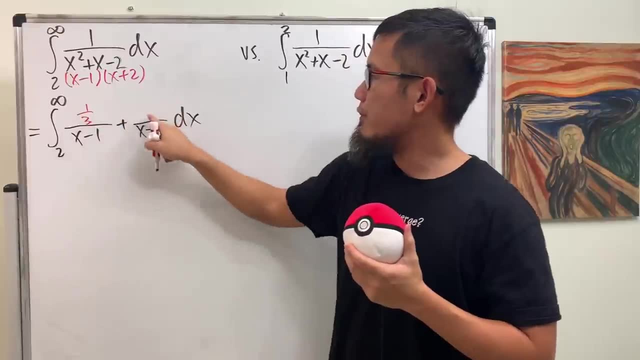 original cover this up, and x has to be 1, and we put it there. 1 plus 2 is 3 on the bottom, so we have 1 third right here. And then, to figure out this, well, go back to the original cover this up: x has to be. 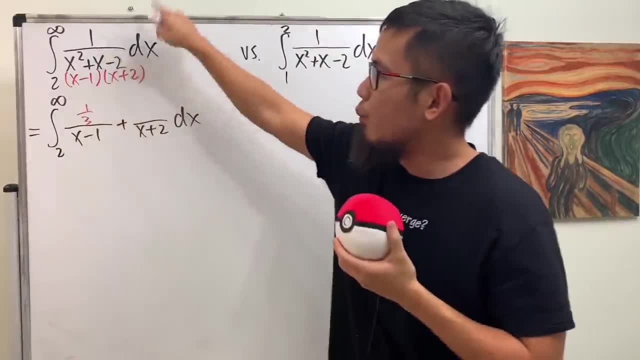 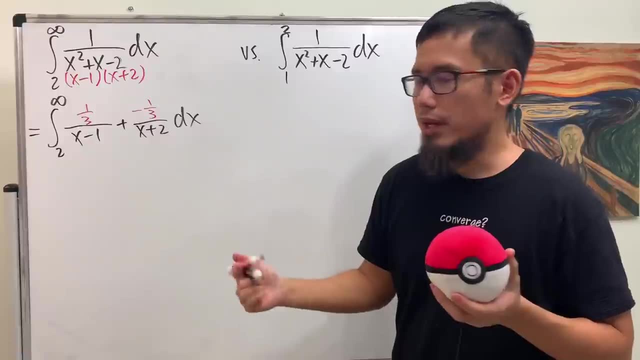 negative infinity. Put it there. so we have 1 over negative, 2 minus 1, so we have negative one-third. So both of them have a third right And this is negative, And we can go ahead and integrate this. 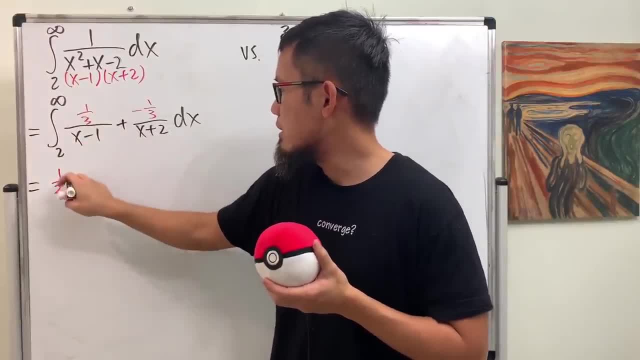 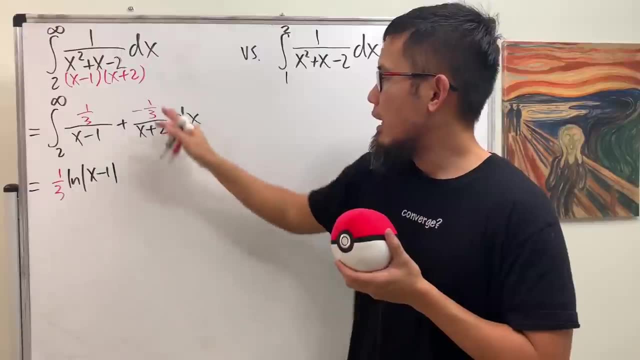 First this right here is one-third, and then natural log: absolute value of x minus 1.. And because this is just a 1, dividing by 1 doesn't change anything. And then next we have minus one-third, Ln: absolute value of x plus f. And then let's wake it up. How do you solve it? One over negative 2★1.. So that's where we take it, Karen. how did you get this? Next, we have x minus one-third divided into the third. First, this right here is one-third, and then natural log: absolute value of x plus one. 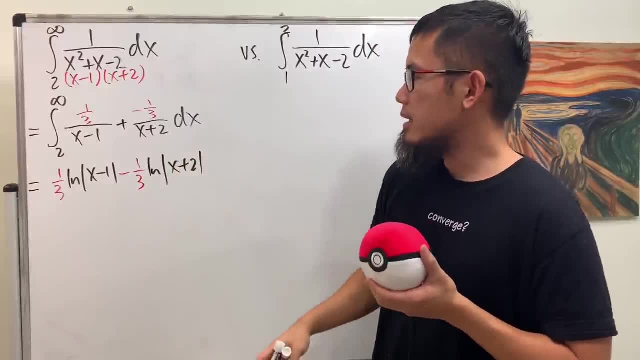 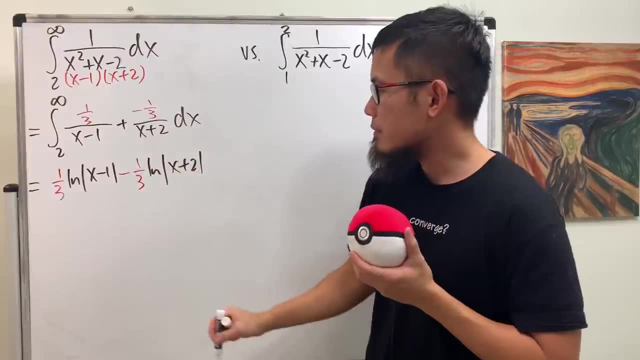 And because this is just a one- dividing by one doesn't change anything- plus 2, and that's pretty much all we have, And I'm actually going to put them together as one single logarithm, and then I will do the 2 to infinity, right? So right here we can factor. 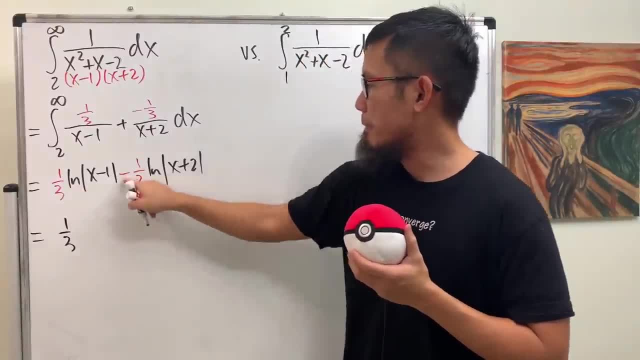 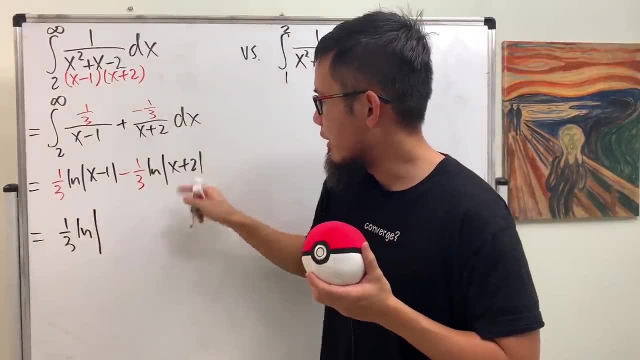 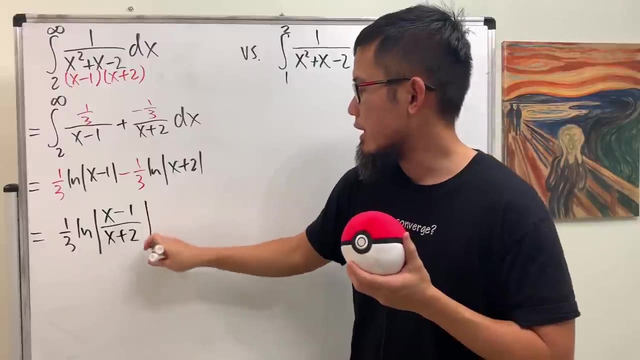 out the 1 third, and because we have this natural log minus this natural log, when you put them together it becomes natural log of the first divided by the second. so x minus 1 over x plus 2, like. so So that's what we have, And then here let's go ahead and plug in 2 to infinity. 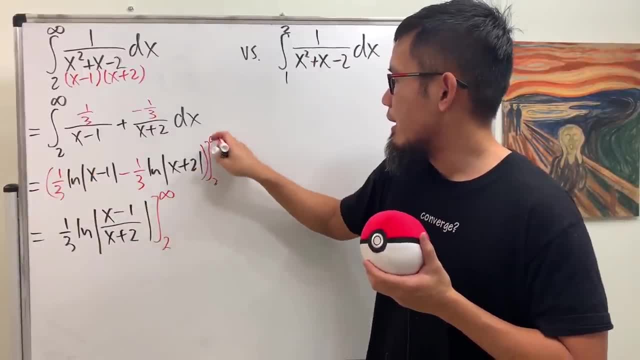 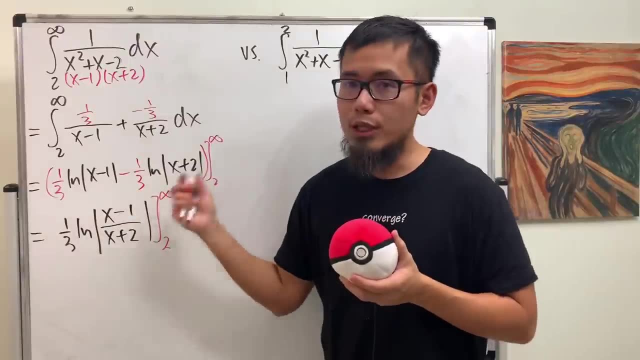 Oh, technically, I should also do that right here. And the reason that you want to do this first before you put in the limit, it's because if you put a limit in here and here, you actually get infinity minus infinity in the same parentheses. Well, in that case, go ahead and combine them. 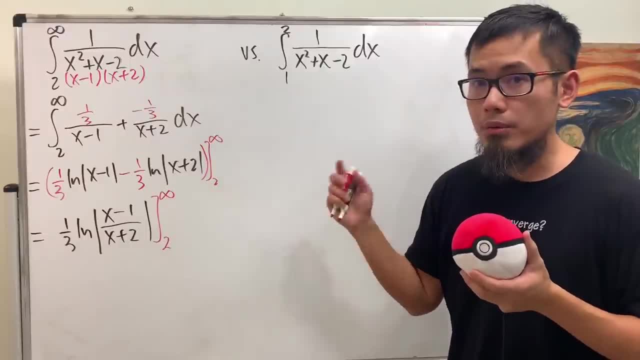 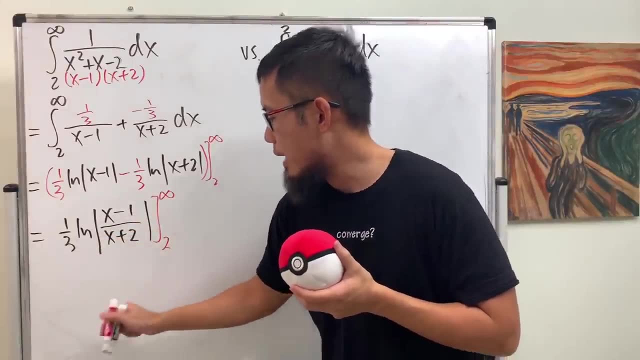 and use the natural log property and do the L'Hopital's rule if necessary. All right, the first trouble is when we put infinity into here. we actually get what, though? Well, I will actually have to show you guys the work on the side, just to be legitimate. We will actually. 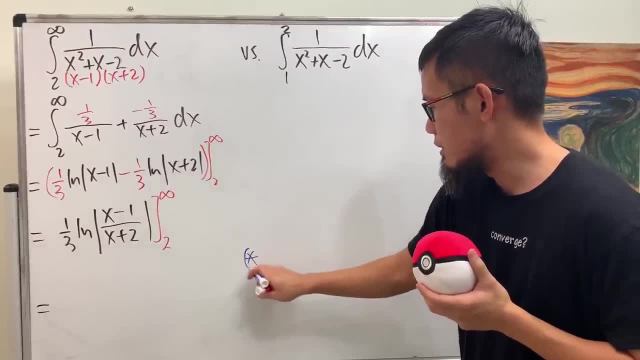 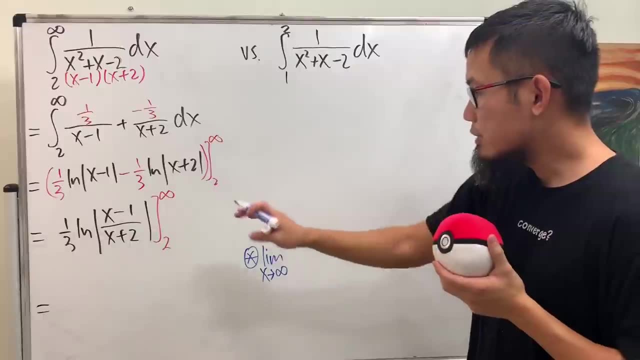 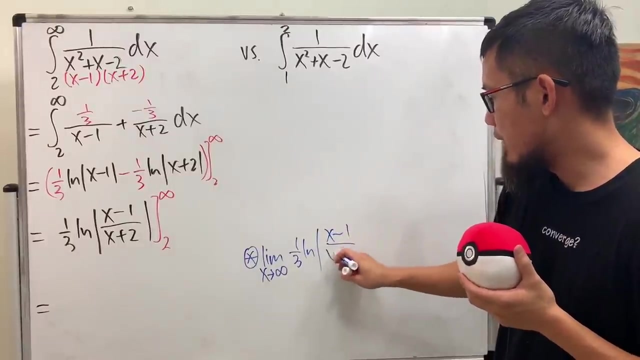 have to take the limit, so I'll just put this down right here. So this is just a blue star. We have to take the limit as x approaching infinity. And let's just look at the first part: 1, third ln. x minus 1 over x plus 2.. 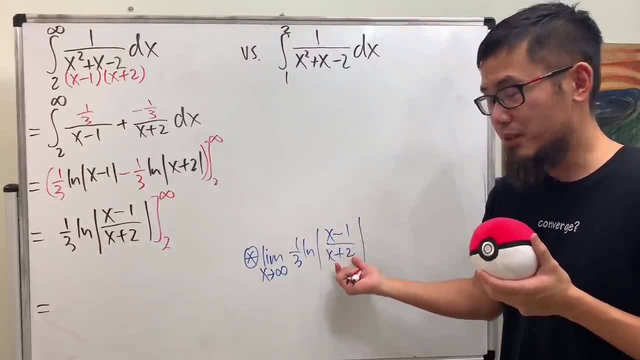 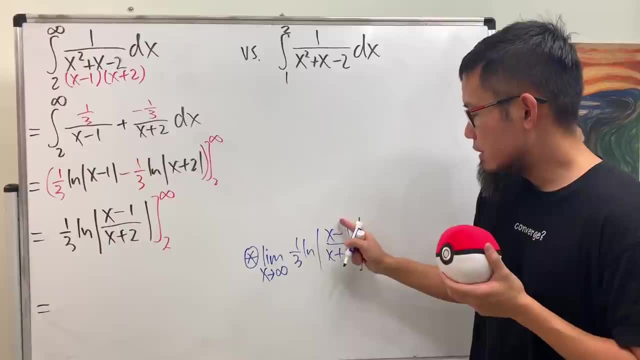 If you put infinity, you get infinity over infinity inside. That's why you have to put it on the side and do more work on that. Well, the truth is, when we have infinity over infinity, in this case, even though it's inside of the natural log, but you can still bring the limit. 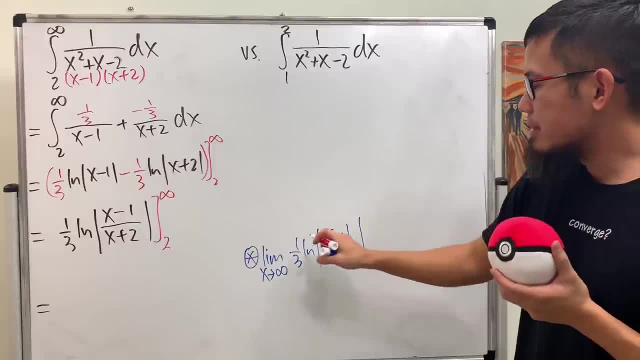 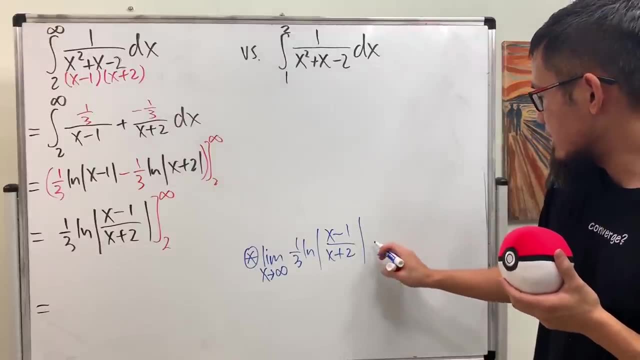 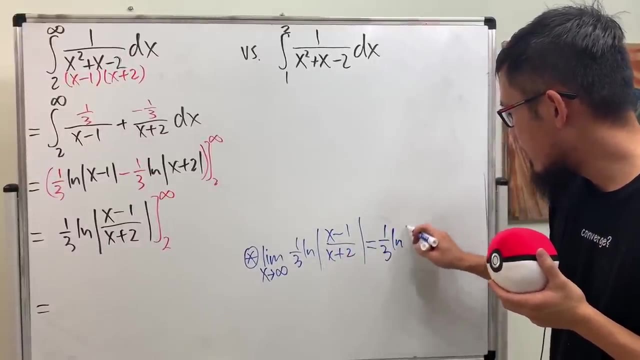 inside and then do the L'Hopital's rule. Why? Because natural log is a continuous function, so you can just evaluate the limit inside. And when you do that, let's see. if I put it here this is going to be: we have the 1 third on the outside, and then ln, absolute value, And again. 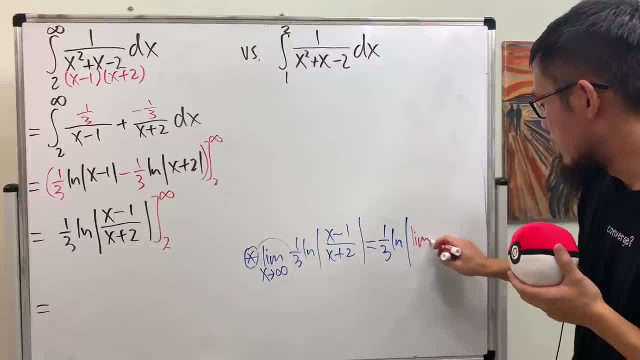 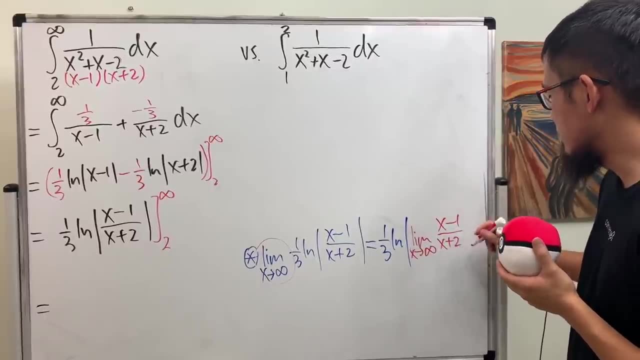 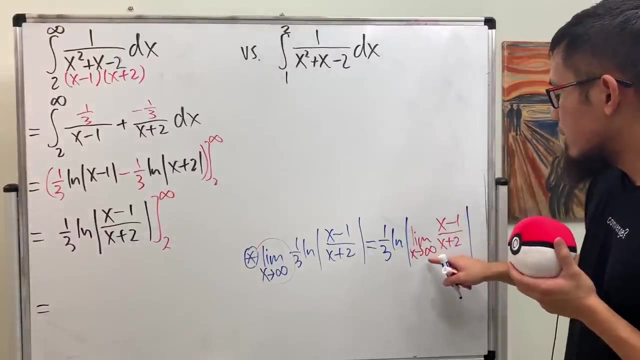 I'm looking at the limit, but I'm putting the limit inside, And then x goes to infinity, and then we have the x minus 1 over x plus 2, like so. So that's pretty much what is happening. You do things inside out And right here. if you put infinity here and here, well, you have two ways to do it. 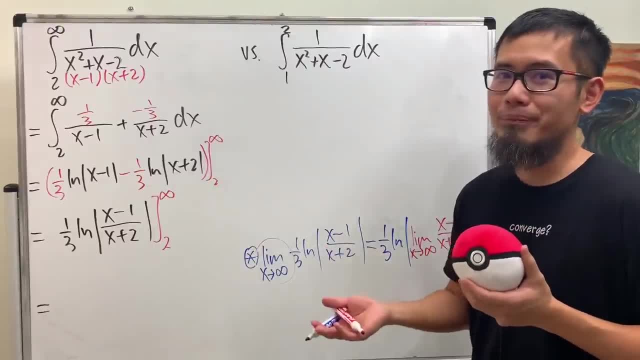 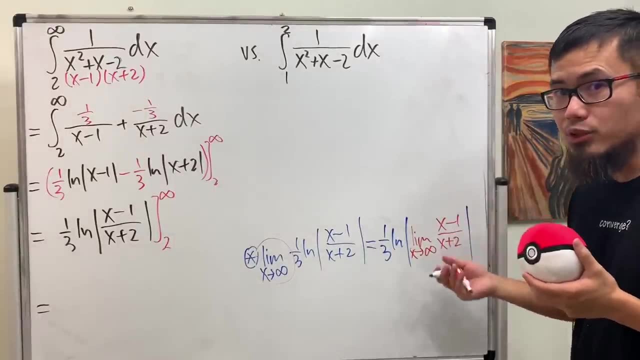 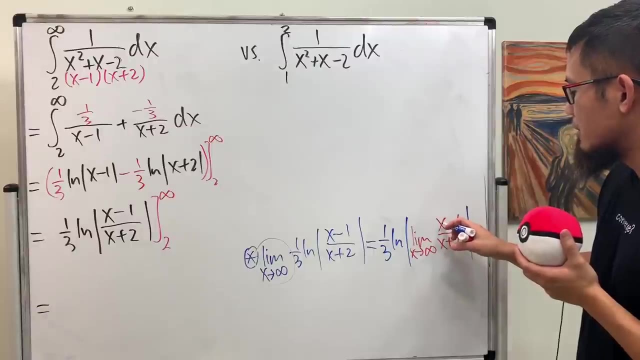 The first way is you can just do L'Hopital's rule. The second way is because we have a power function over a power function or polynomial. technically, you can just pay attention to the dominating part of the top and also on the bottom. Well, technically, right here it's just going to be. 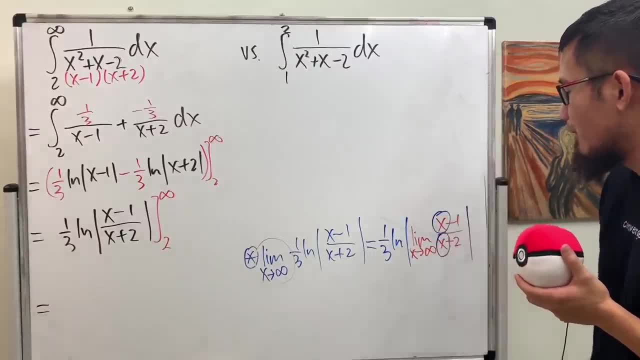 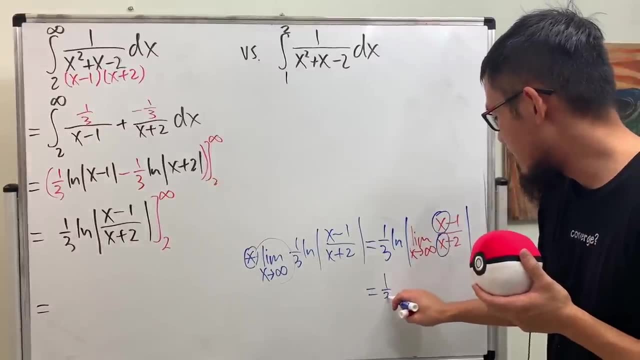 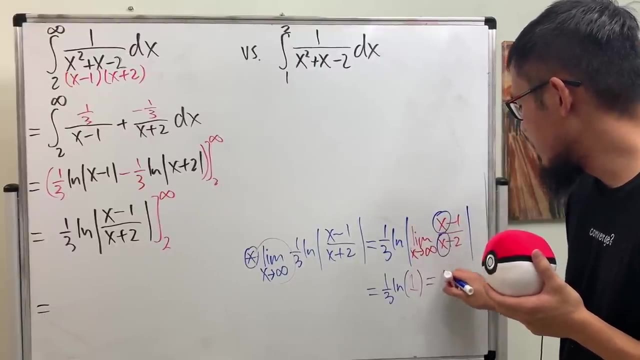 the highest power of x And because they are both x to the first power. so you see, this is just going to reduce to be 1.. So all in all, this gets to be 1, third ln. the limit of this is just going to be 1.. So we have ln of 1, and then this is going to be 0,, right. 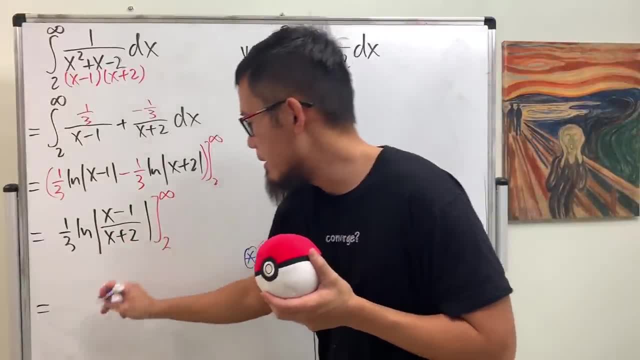 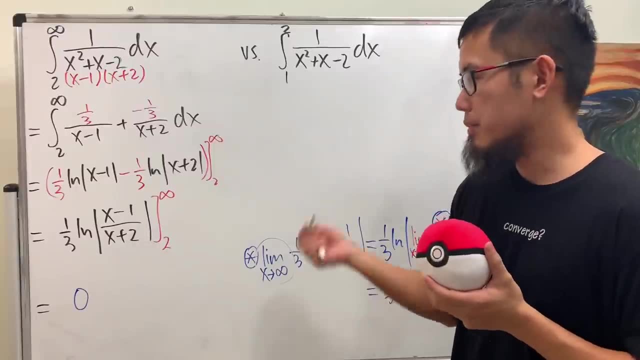 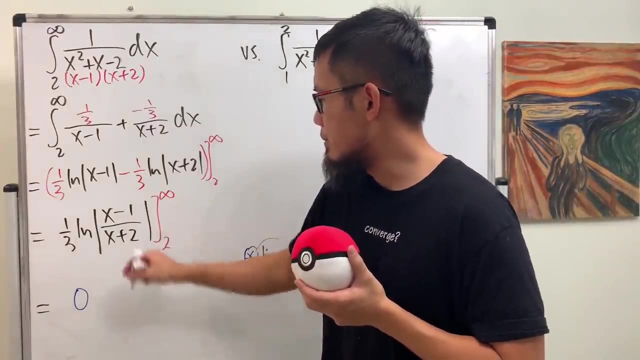 Therefore, when we put the infinity to here, it's legitimately equal to 0, and you can just, you know, supply your work on the side, especially on the x-axis or so, because otherwise you just have to do things carefully. Anyway, to continue, we plug in 2.. So we have 2 minus we have. the second. one is 1, third. 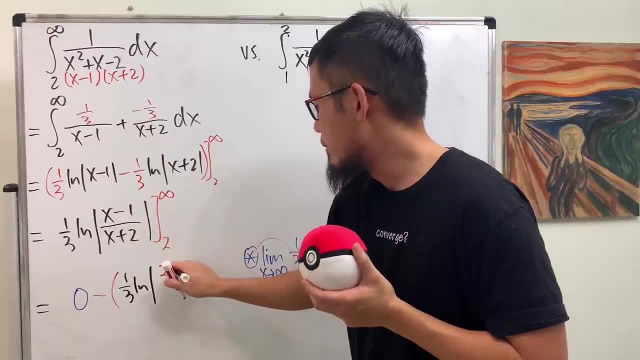 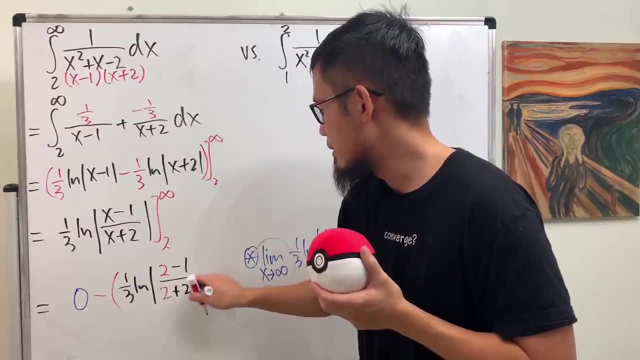 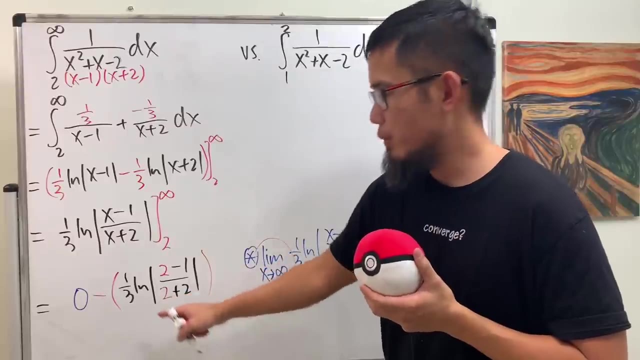 ln absolute value, putting 2 in there: 2 minus 1 over 2 plus 2.. So here we have 2 plus 2, like: so Alright, so now this is 1 over 4, and then we have pretty much 1 third and all that stuff. 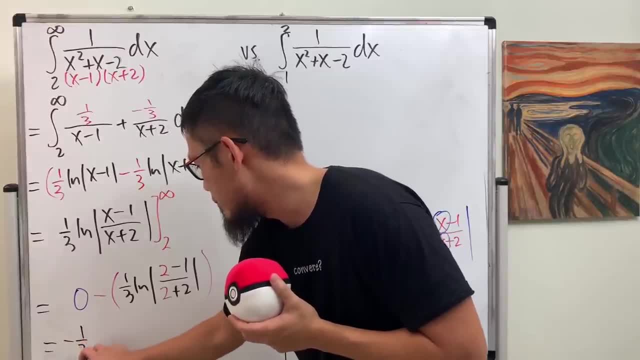 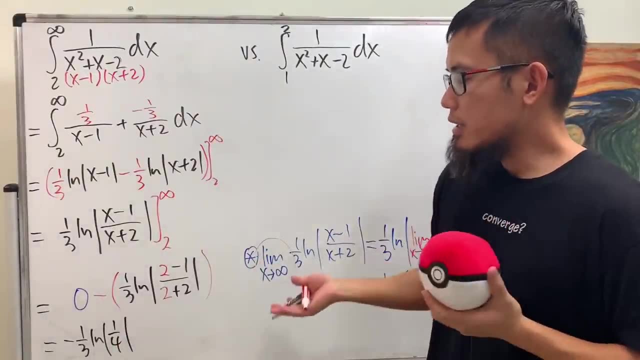 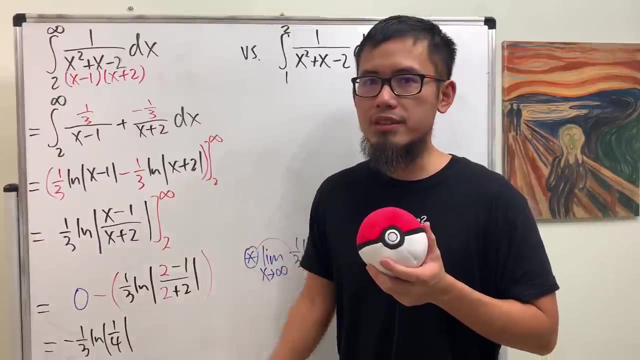 So, all in all, here we go. This is negative: 1 over 3, ln of 1 over 4, like this right. Actually, it's the final value. so that means this right here converges. and the truth is, let me ask you, is this a positive or negative number? 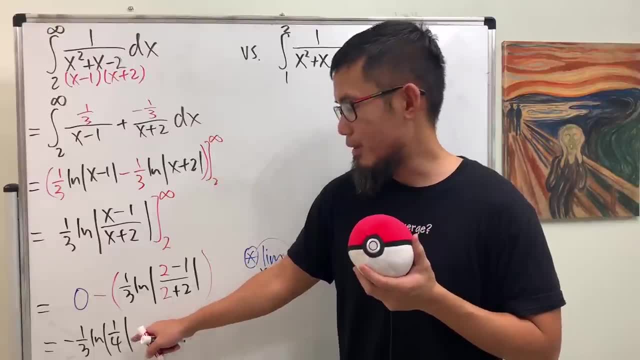 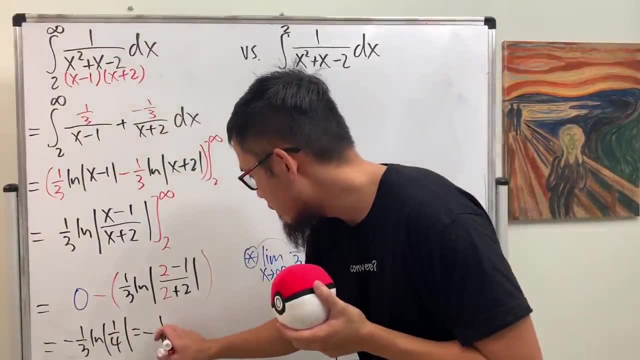 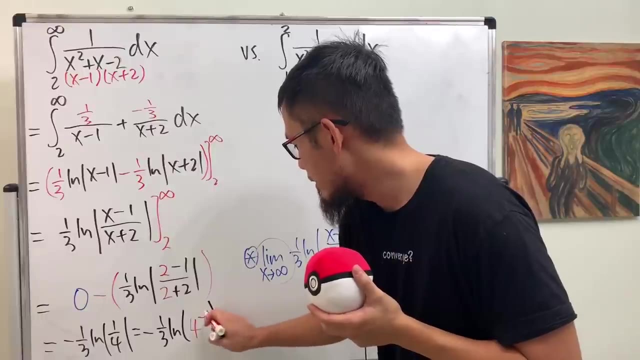 This is actually a positive number Why? Because if you look here, 1 over 4 as 4 to the negative 1 power, this is 1 third ln of 4 to the negative 1 power. you can bring the power to the front. 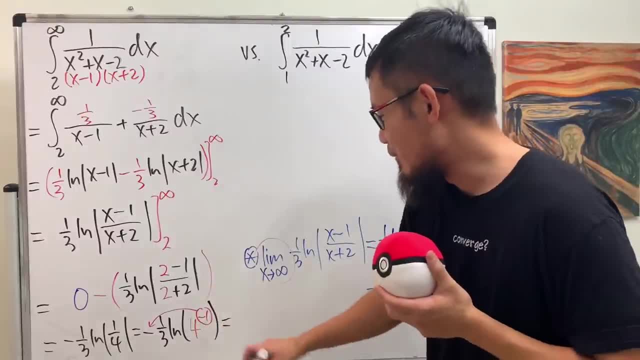 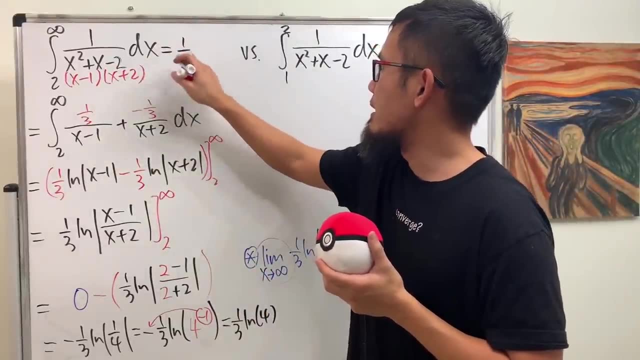 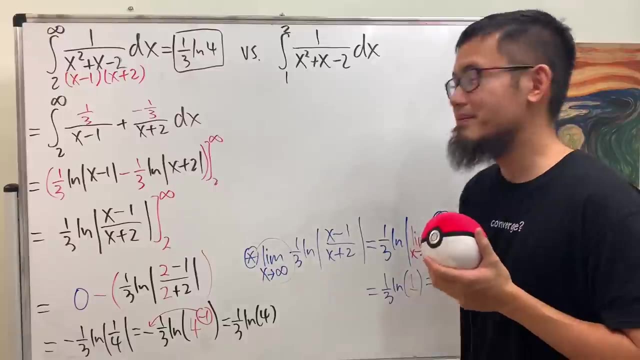 and that's not power rule. so just don't subtract one, you actually get a one third ln four. so this, right here, is the answer. i'll leave it like that: one third ln four. so natural, convince you guys that that is positive, right? because remember, ln if the input is in between of zero and one, you get a. 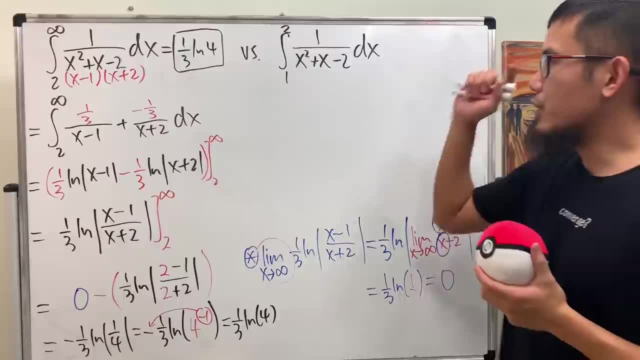 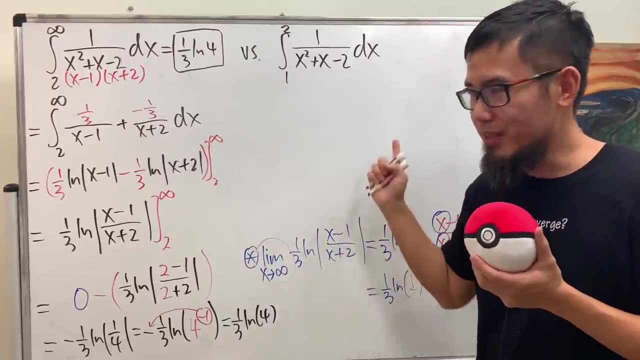 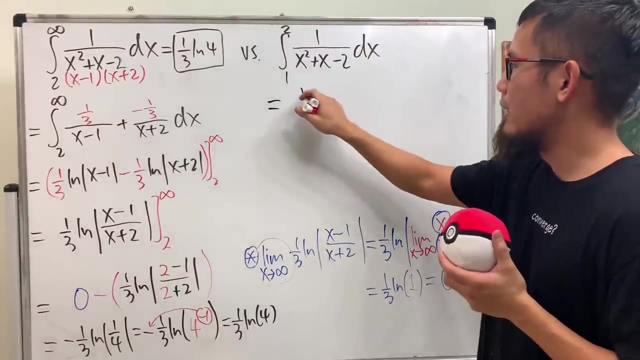 negative output. all right now for second one. maybe you can take a guess if this converge or diverge. that one converges already, though how about this one? well, let's just go ahead and do the work. you don't have to repeat the same integration, so i'll just put down the result right here. this is one. 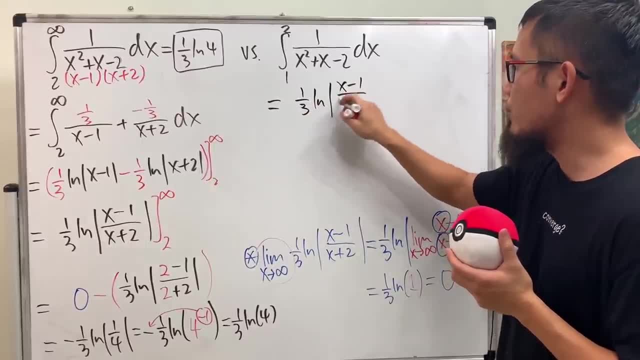 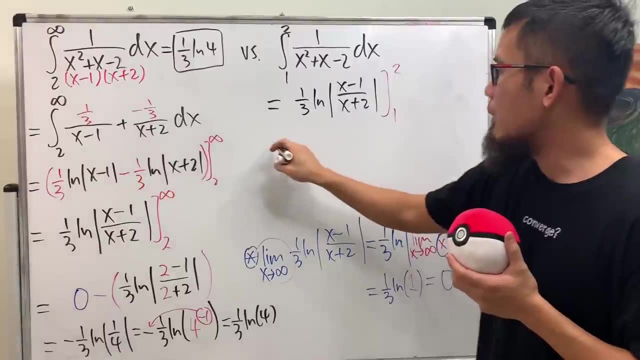 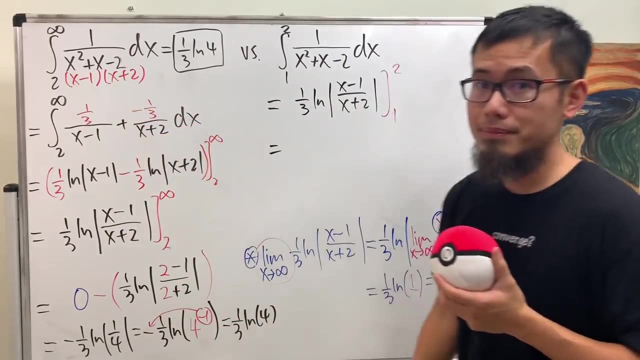 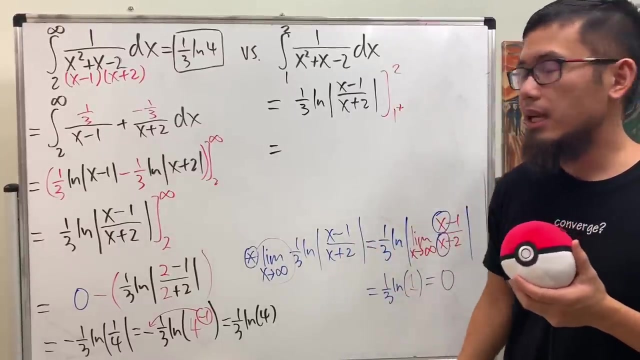 third, ln absolute value, x minus one over x plus two, and we have going from one to two this time. all right, putting two and putting one, but remember what we talk about. if we have x is equal to one. right here you, this will have a vertical isotope. so right here this is technically one plus. and if you wonder, 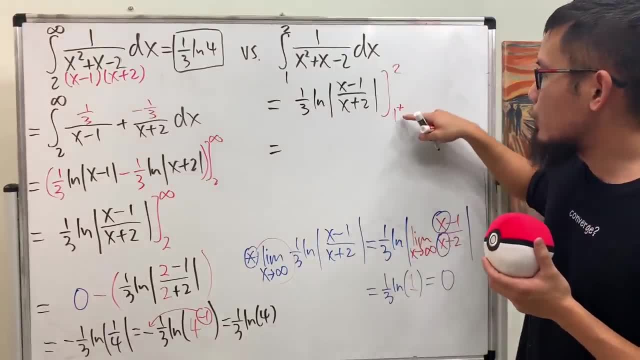 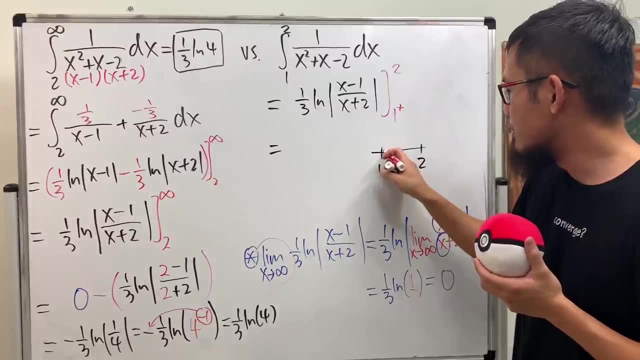 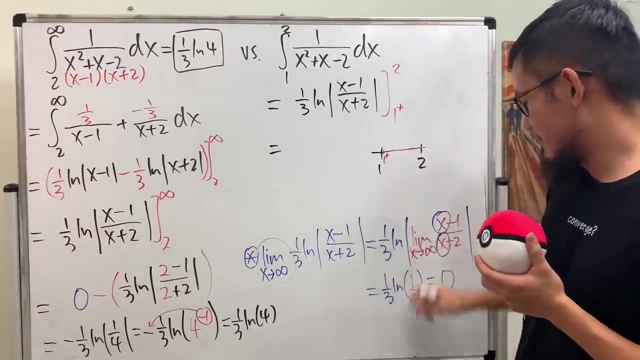 why is one plus one or one minus? because you're going from one to two. right, you're going from one to two and you have to avoid one, and to do so you just have to stop a little bit. right, just a little bit before one. so this is one plus up to two. yeah, just like that. that's why. so that's. 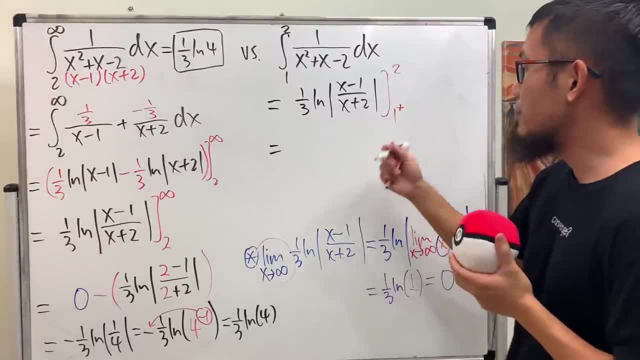 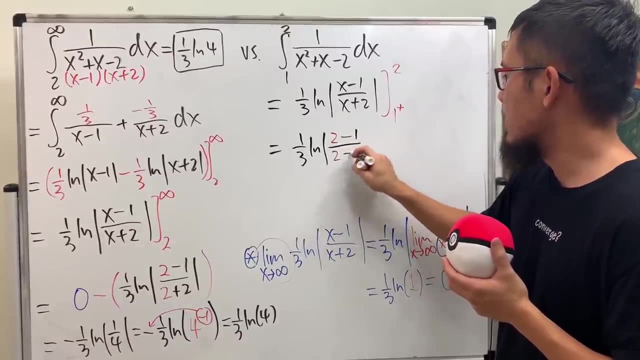 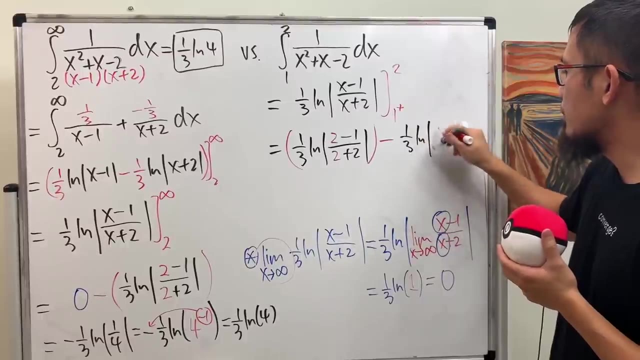 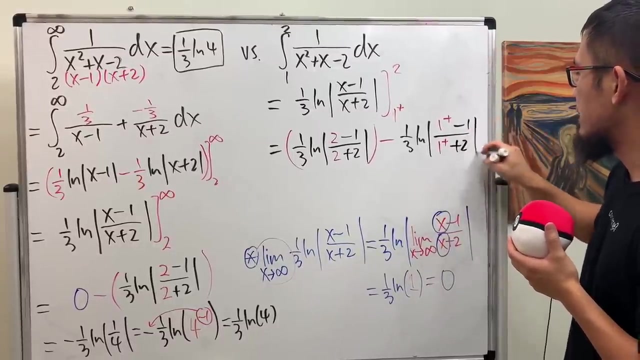 an idea, all right. so putting two and putting one plus and see what happens: one third ln absolute value two minus one over two plus two. that's the first part, and then minus m we have one third ln absolute value one plus minus one over one plus plus two, like so. 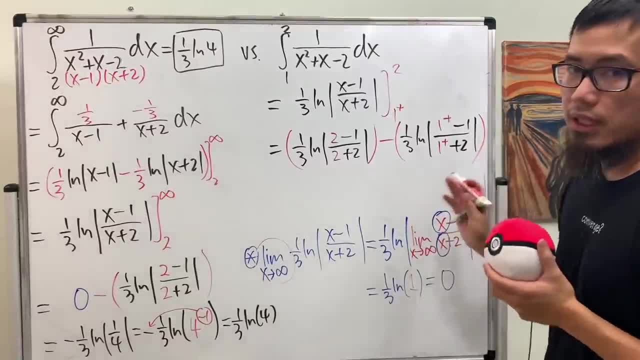 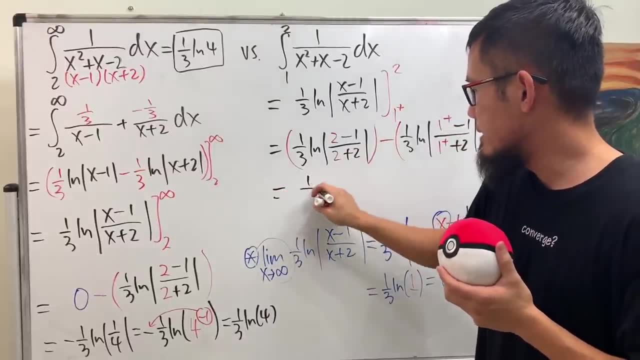 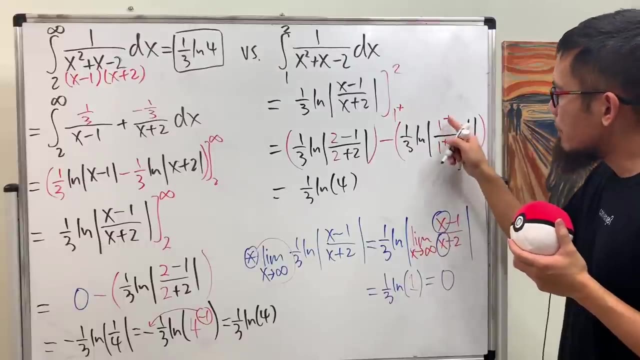 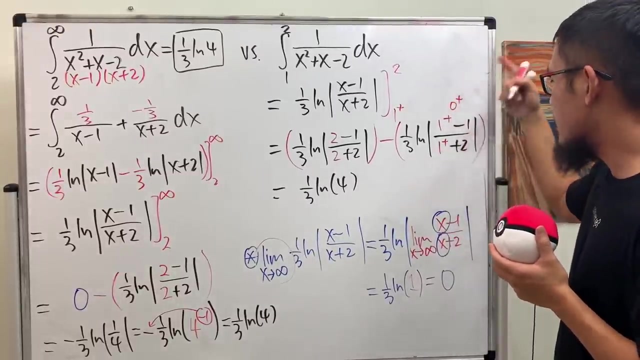 all right, let's see if we can draw a conclusion on this one or not. this right here is this right. so we know it's just going to be one third ln four. so that's great. but for this, if you focus on the inside, one minus my one plus minus one, this is zero plus, and zero plus divided by whatever is still just going to be. 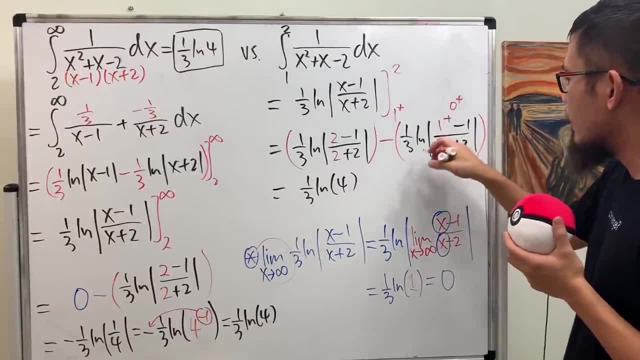 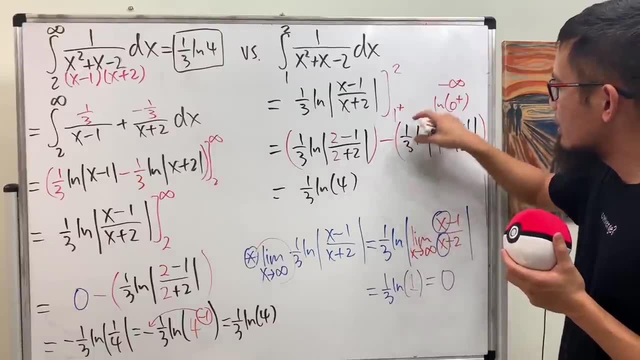 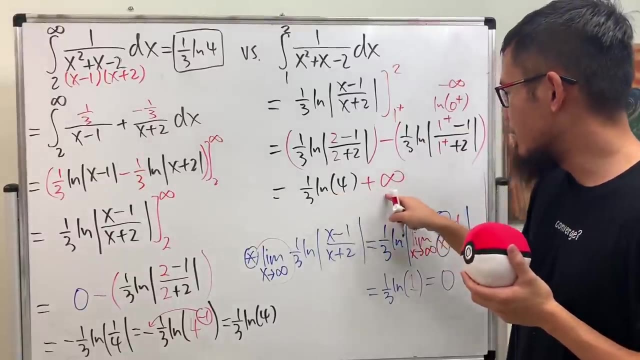 zero plus especially, this is just a finite number. so you are really looking at ln of zero plus and we will end up with negative infinity, negative, one third times negative infinity. we end up to get plus infinity here. so this right here is finite plus infinity. oh wow, this turns out to be infinity. 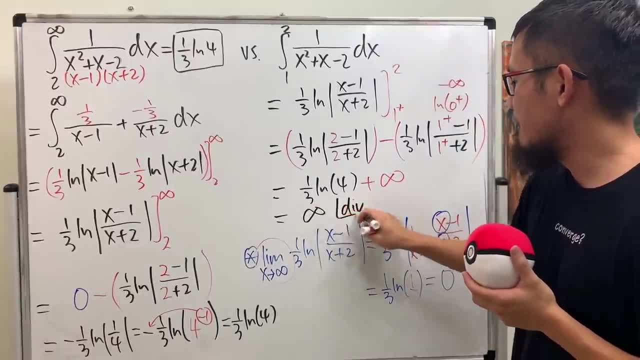 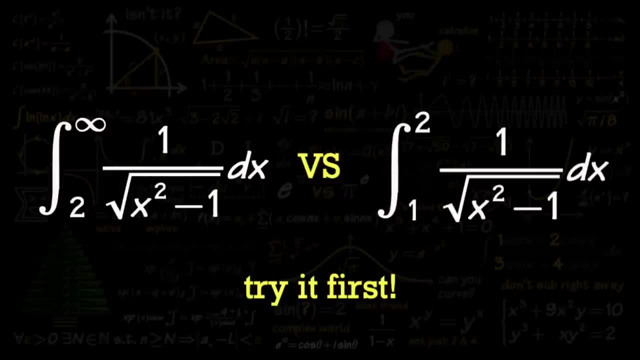 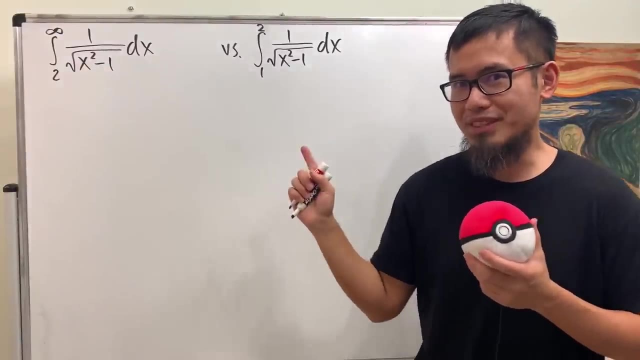 so in this case, right here, it actually diverges. notice that this time we have square root of x, square minus one on the bottom. don't do partial fractions because we have the square root right, but here we can actually do tricks up and the correct substitution is: 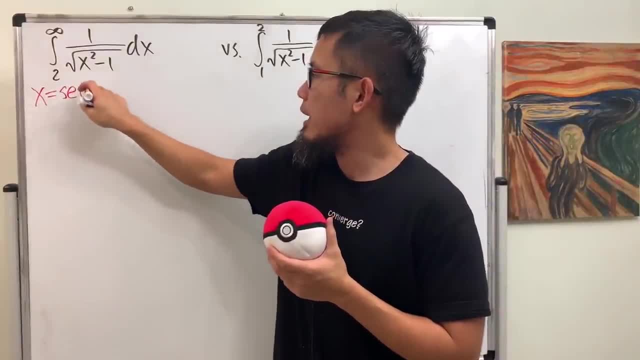 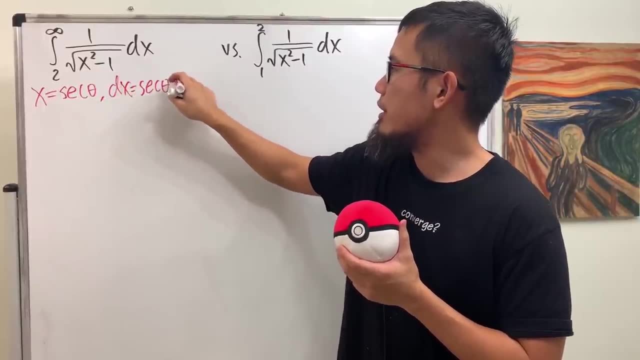 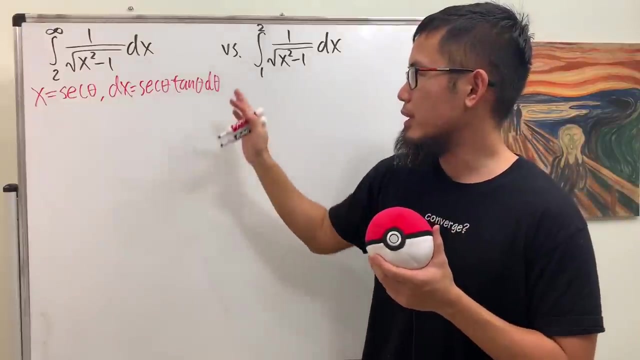 let x to be secant theta right. and then you see that this way, dx will give us secant theta, tangent theta, and of course you have the d theta right here. perfect. now go ahead and just plug in everything into the original integral, and it depends on how you want to do it. you might want to finish everything in the 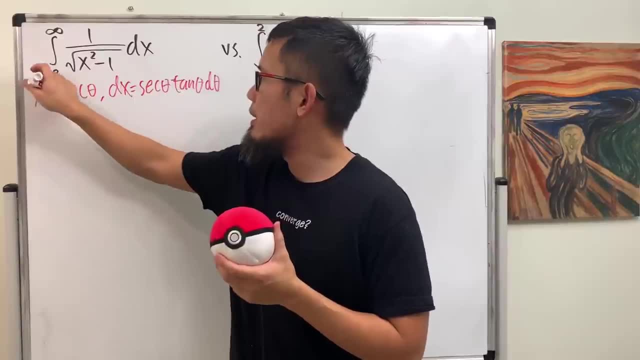 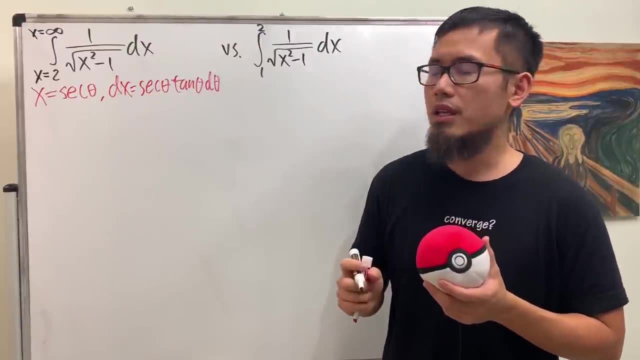 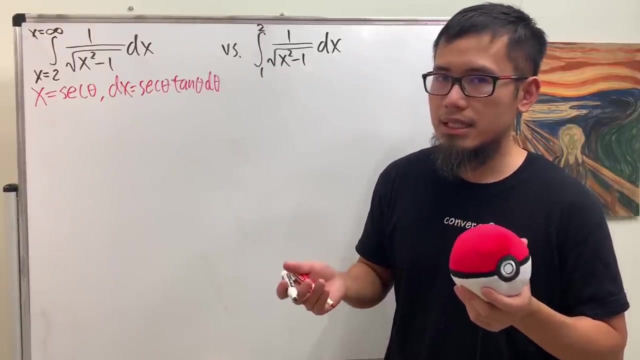 theta world. and if you want to do that, well, here is x is equal to two and here is x is equal to infinity. so you have to just do this one very carefully and it's up to you- right, it's really up to you- to see if you want to work out the trick or not. I will not. 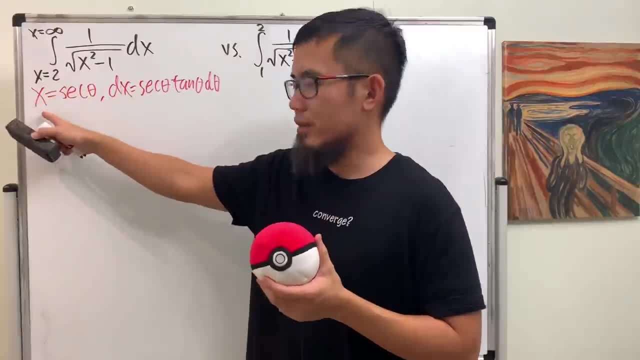 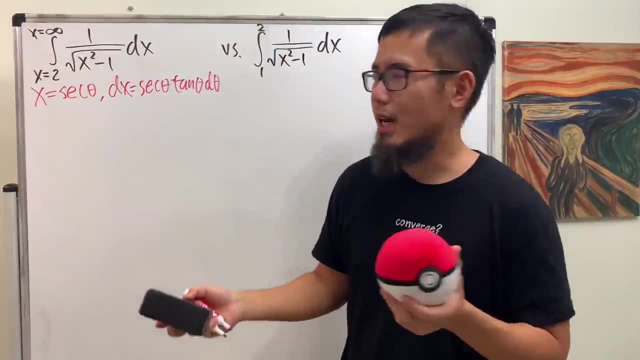 do that actually? because if you put two right here, the first question that you get to ask is that how do I solve secant theta is equal to two? likewise, if you put infinity right here, you ask, like how do I solve secant theta is equal to? 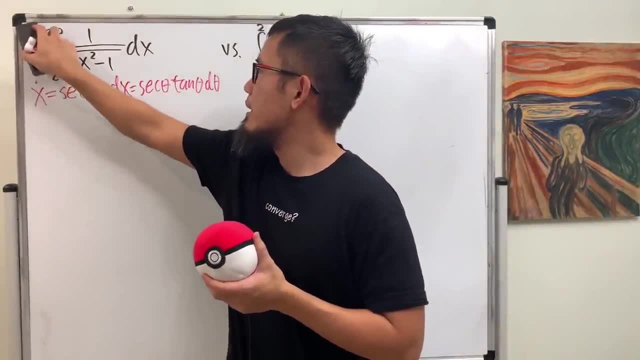 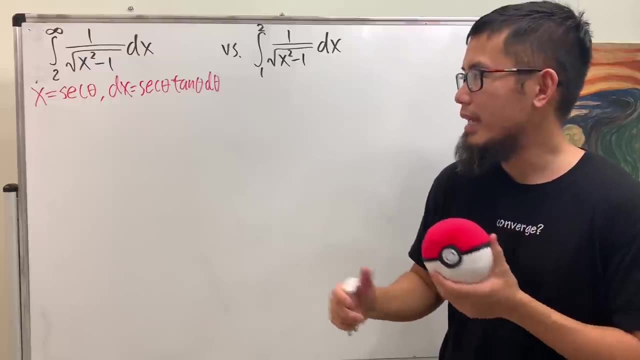 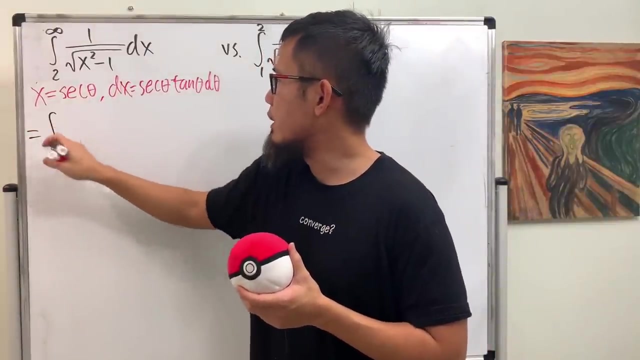 infinity. right, it might be better if we just use tricks up, just go to the theta world to finish the integration and then come back to the X world and then do everything here. so let's just ignore the numbers right here for now. so, with that being said, let's just focus on the integration. here we have 1 over square. 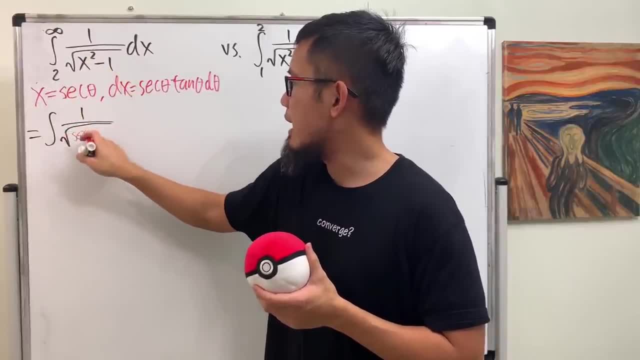 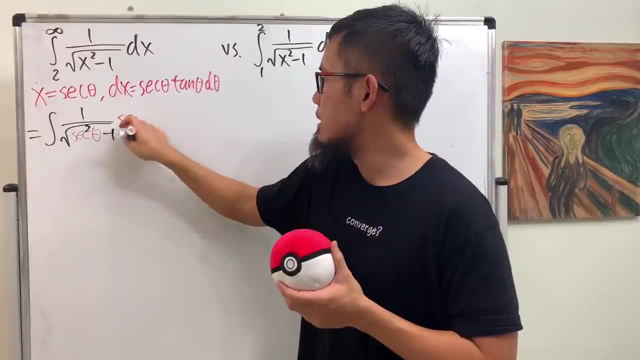 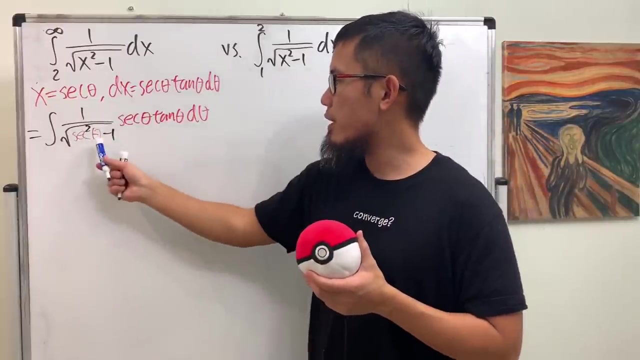 root of and this right here is secant theta, and we have that being square, and then we have the minus 1 and the DX is all that. so I'll just write down secant theta, tangent theta, d theta, like: so, all right, what's secant square theta? 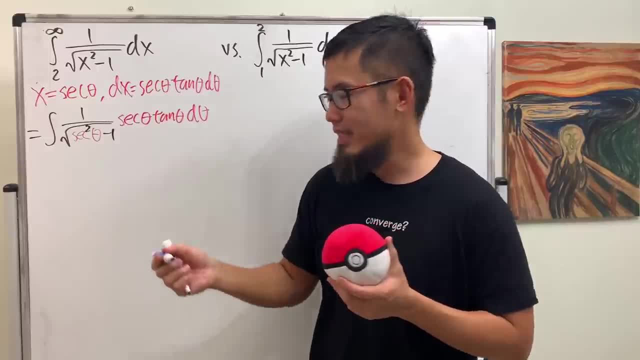 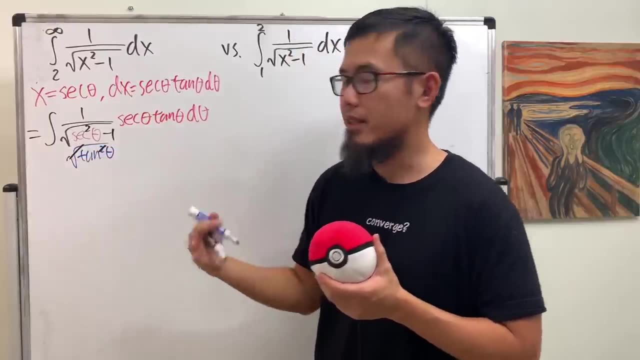 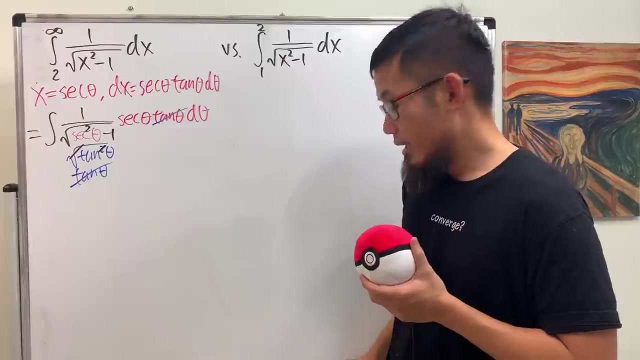 minus 1 tangent square theta. right. so this is just square root of tangent square theta and, yes, they will cancel. so we have a tangent theta on the bottom and the best part is this: and that will also cancel. in another word, we just have to integrate secant theta. so this right here is the tangent theta and this is the. 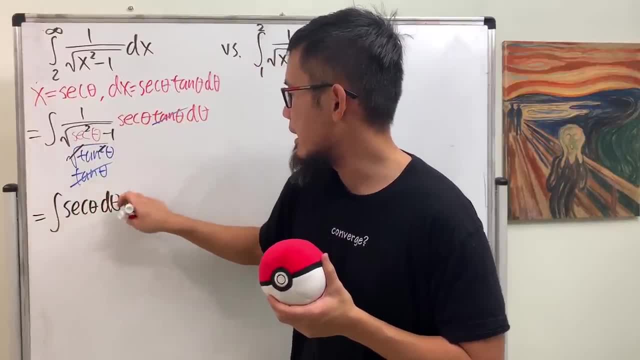 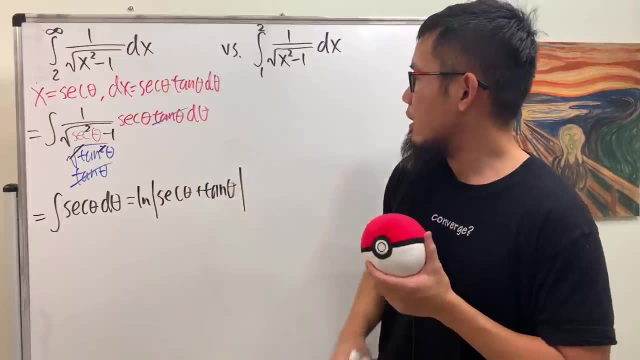 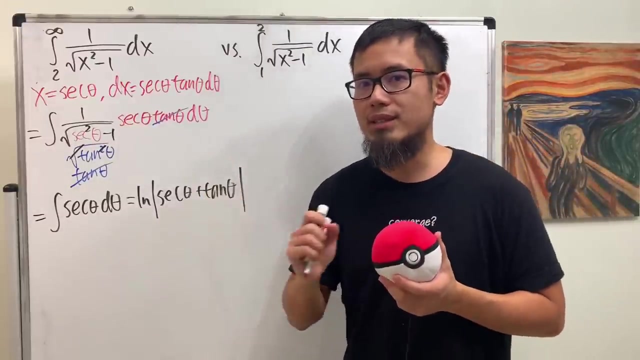 right here is the integral of secant theta, d theta, which is going to be LN, absolute value of secant theta plus tangent theta. don't worry about plus C, because we are going to plug in numbers, but we do have to worry about going back to the X world again. that's just my recommendation, especially when you are 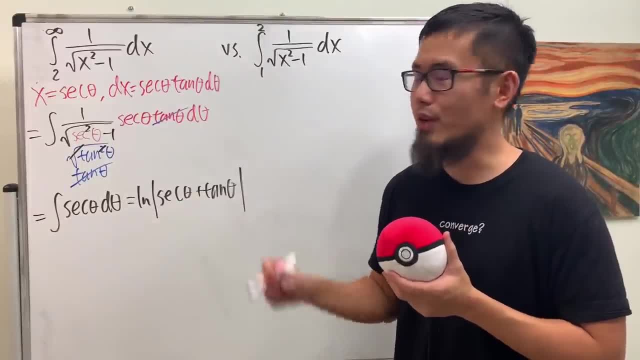 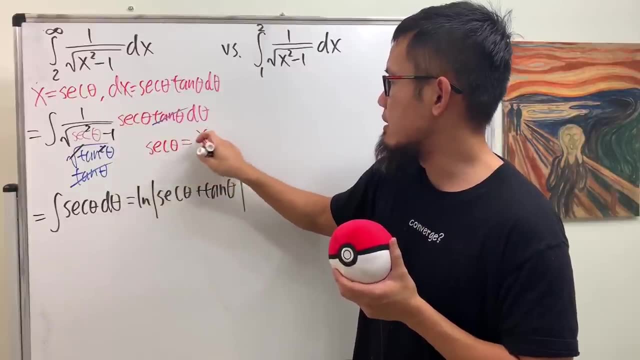 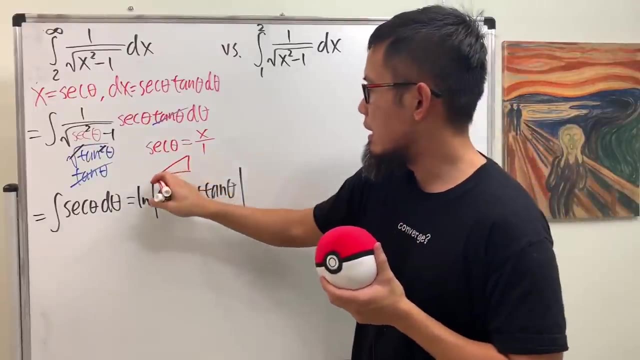 doing the trig substitution, go back to the X world and then work on the numbers there. well, we know that secant theta is equal to X, so we can write this as secant theta equals X over 1 and then draw the right triangle and remember secant is. well, let's put on the right angle here and 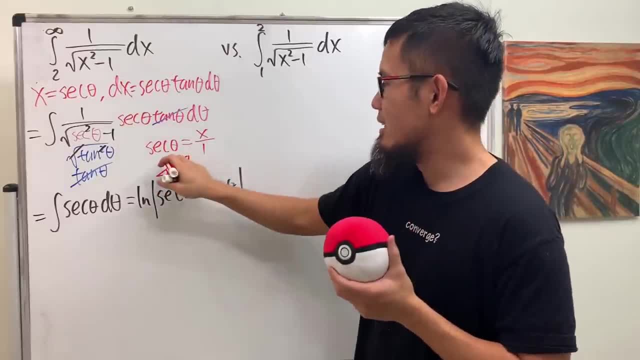 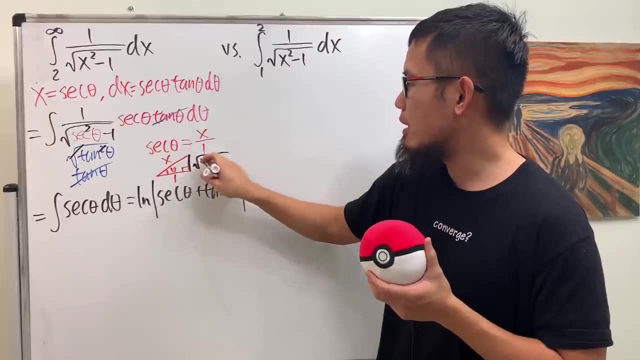 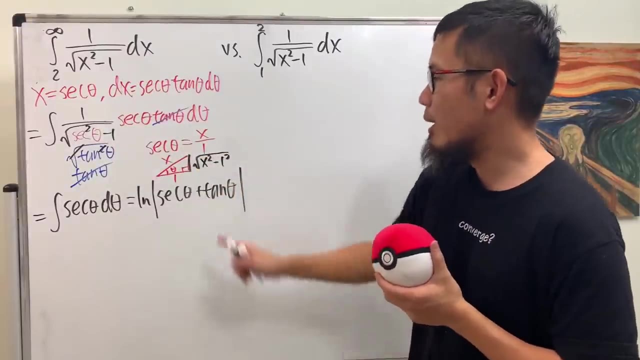 then the angle theta secant is what hypotenuse over adjacent. and the opposite is you open the square root first and you do the hypotenuse square minus this side square, and yes, do you see the same radical again? yeah, alright. so based on this triangle, 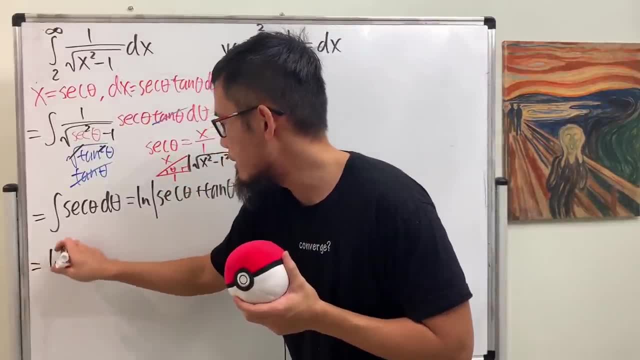 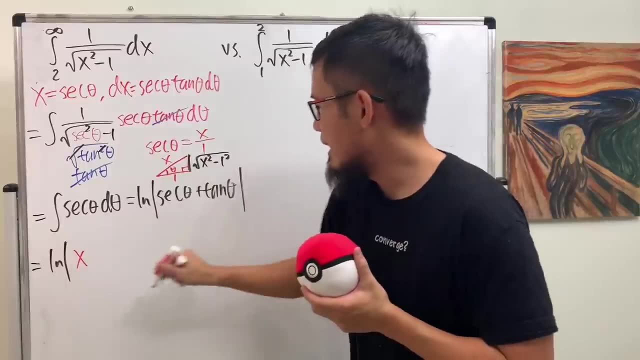 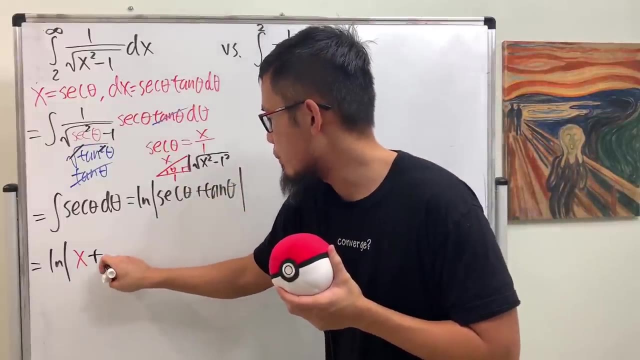 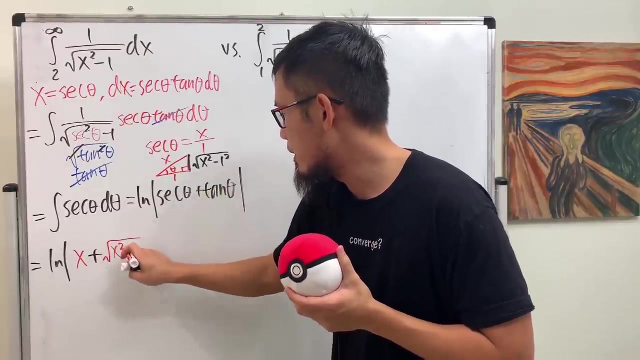 let's go ahead and figure this out. this is LN- absolute value. secant theta is just going to be X, right, that's the next one. good, and then plus tangent theta. well, tangent is opposite over adjacent, so we have just square root of X square minus 1 over 1. so this over that. so we have this X square minus 1, alright, so that's. 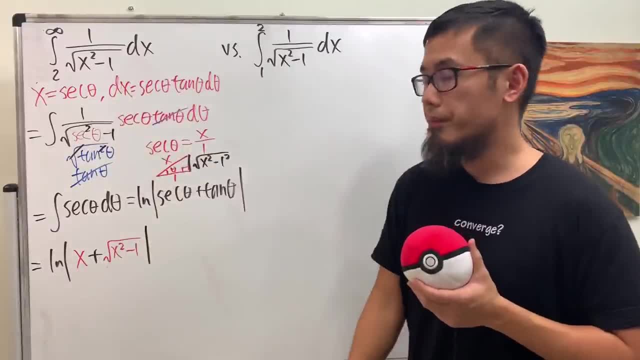 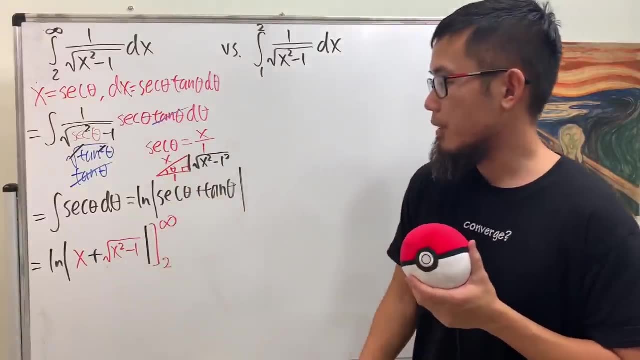 actually our answer to this question. so thank you so much for watching and I'll see you in the next video For that integration. and then we just have to plan Numbers. so let's go ahead, we are going to plug into and then infinity. we've plugged's infinity. 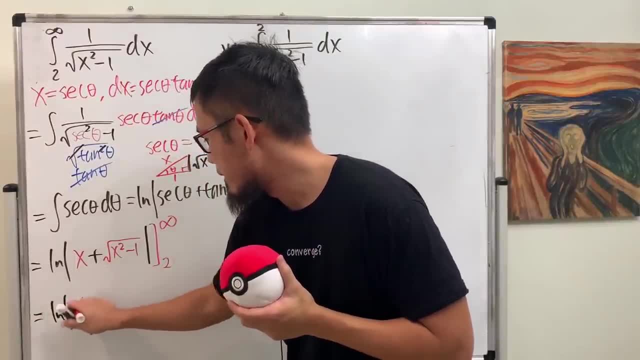 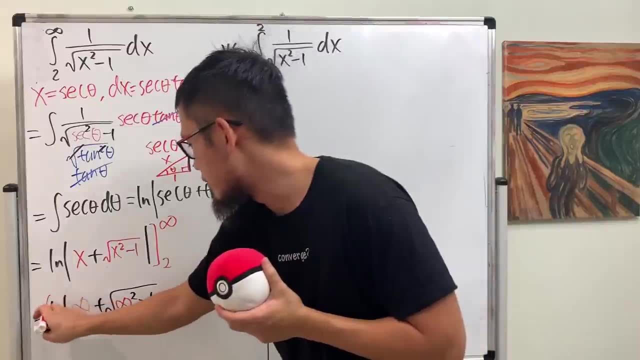 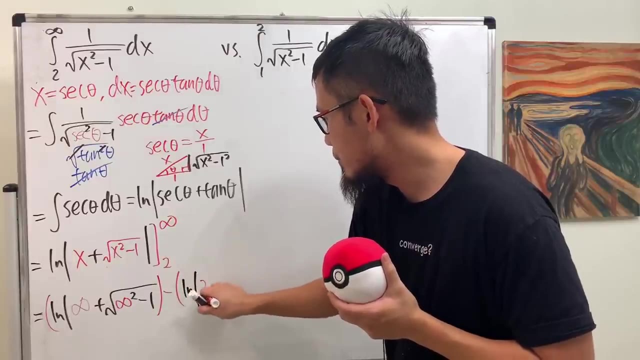 We get natural log of infinity plus square root of infinity square and then minus 1. so this right here is the 1st part. minus Site X, 2, so 2 x, we have LN absolute value 2 plus square root of 2 squared minus 1, just like that. 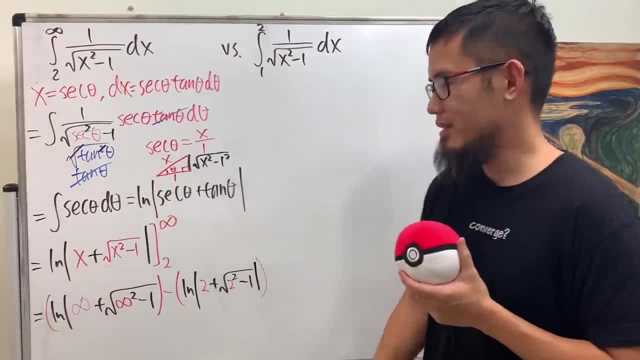 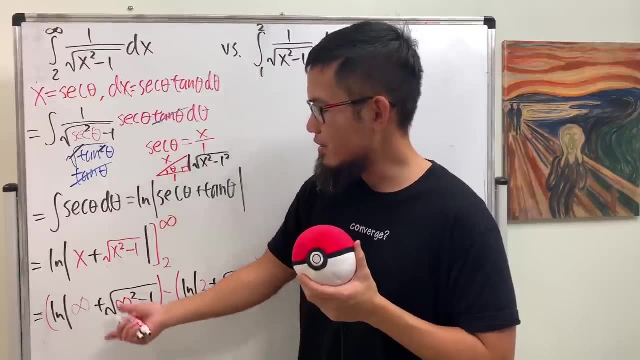 Again, we don't need the absolute value though, because But we can have it, it doesn't really matter, And you know what's happening. This is infinity plus, This is infinity minus. 1 is still infinity. Square root of infinity is still infinity. 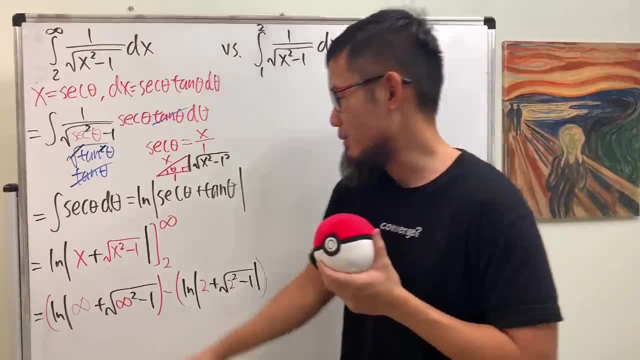 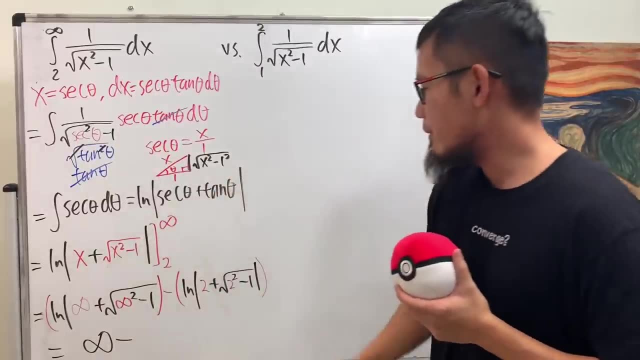 You can make it wrap with the sum of all that already. But anyway, ln infinity is infinity. So the first part here is infinity. Second part is: Well, it's a number, it's a finite number. Remember ln of 2 plus square root of 3.. 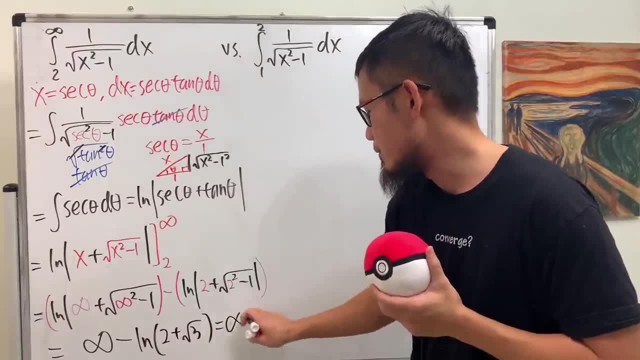 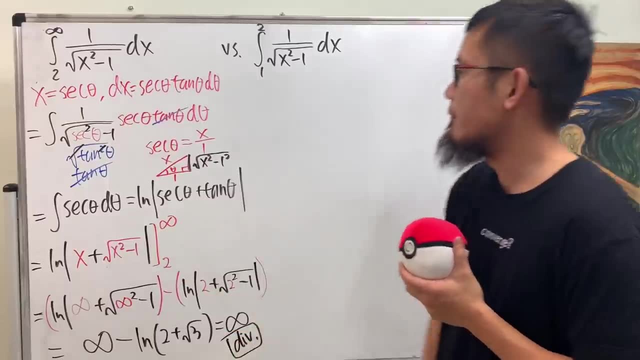 So infinity minus that. The infinity, unfortunately, will overtake that. So this right here diverges, So I'm just going to write it down right here for you guys. All right, We did the hard work already, though, because we used the trick sub to get the integration right here. 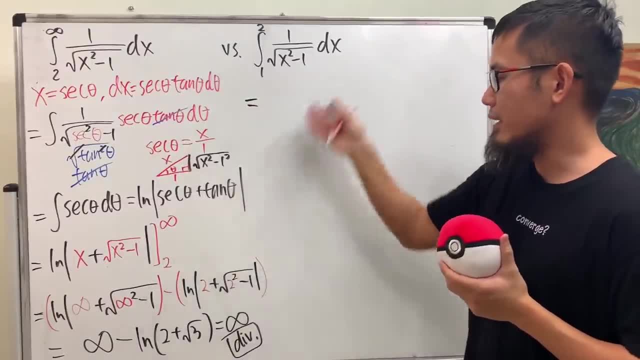 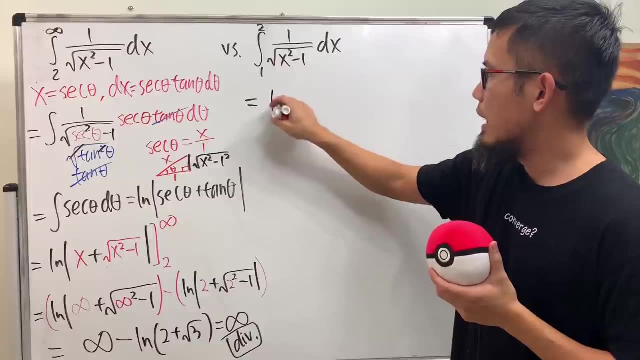 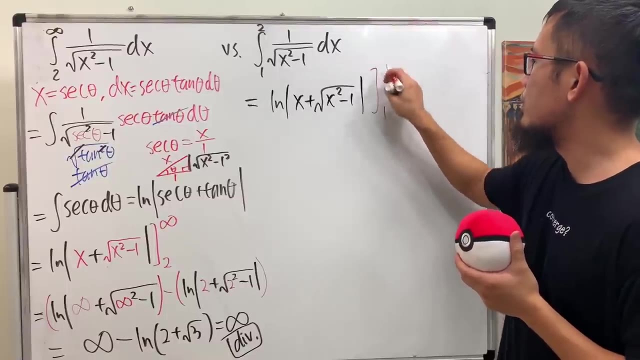 So we'll come back here and do the same thing. Let's just use that and then put it down and then figure it out, Well. Well, this is ln absolute value of x plus square root of x, squared minus 1.. And then we have to go from 1 to 2.. 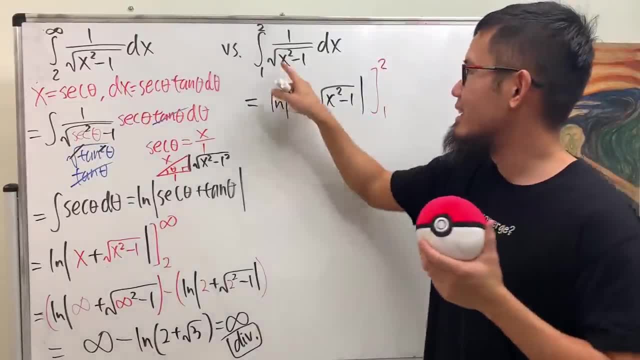 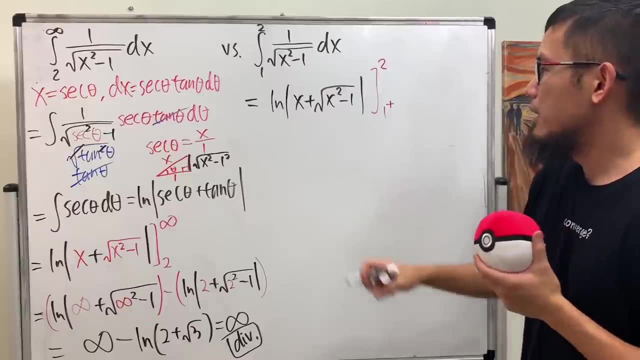 And here we are going from 1 to 2.. But when x is equal to 1, that will give you a vertical asymptote, So the technicality here is 1 plus 2.. But anyway, though, go ahead and plug in. 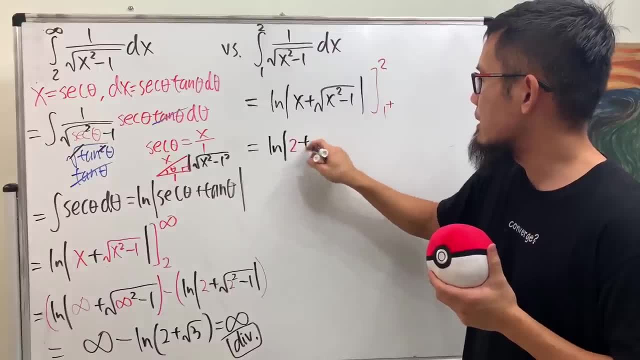 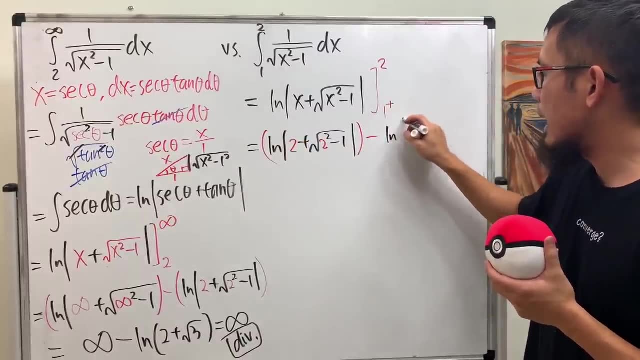 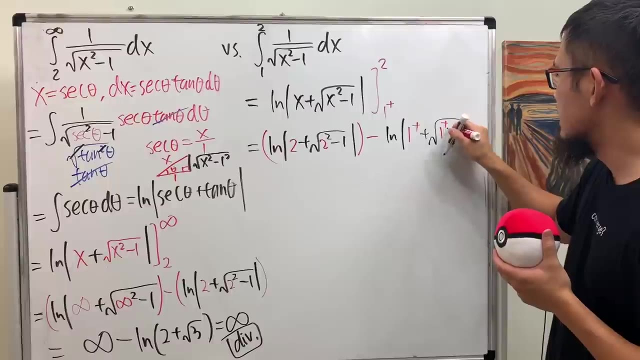 So you get ln of 2 plus square root of 2, squared Minus 1.. That's the first part, And then minus ln, absolute value, 1 plus in there, And then plus square root of 1 plus square And then minus 1, like so. 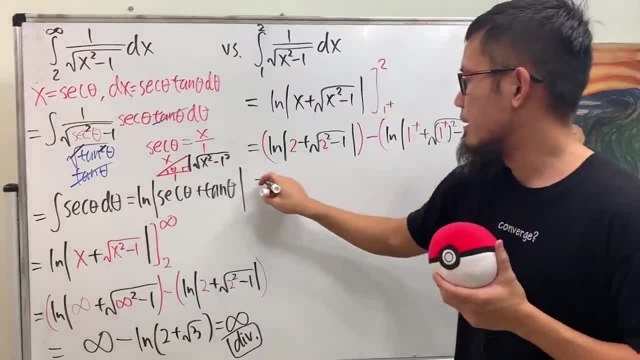 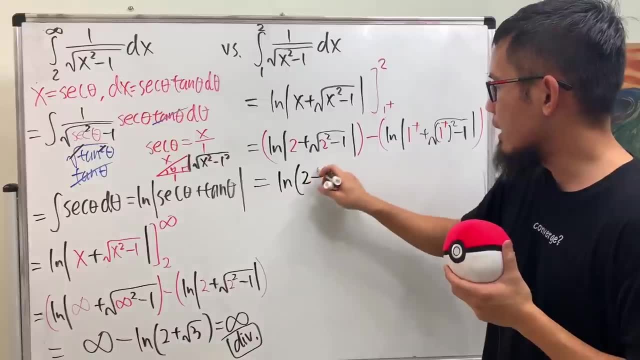 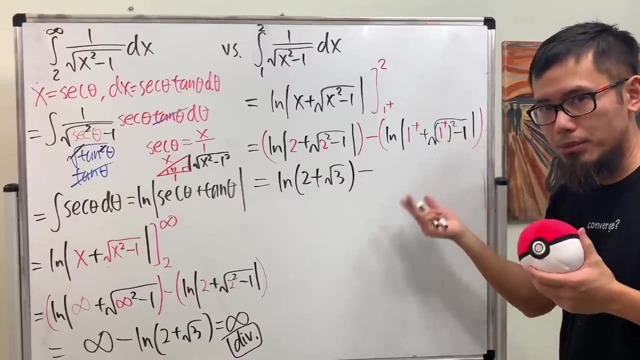 All right. Okay, The first part we get ln of the inside is positive. That's why I changed to parentheses. This is 2 plus square root of 3. And then minus. Have a look: 1 plus square is still 1 plus. 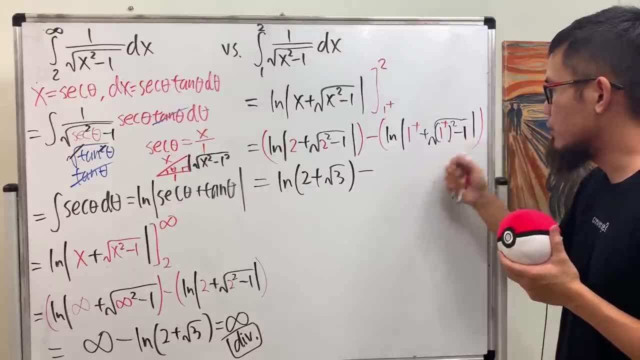 It's like 1, right, And then minus 1 is 0.. Square root of 0 is 0. In the end you get ln of 1 plus, which is like ln of 1.. So all in all, this right here is just 0.. 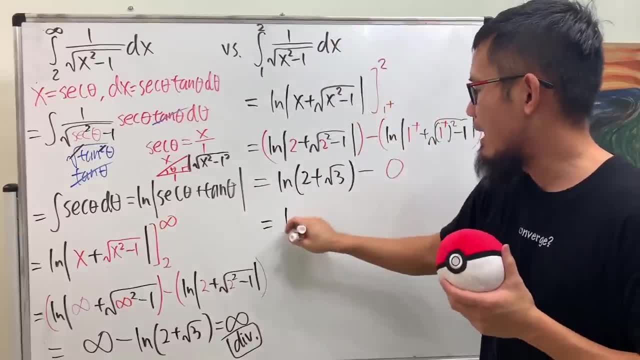 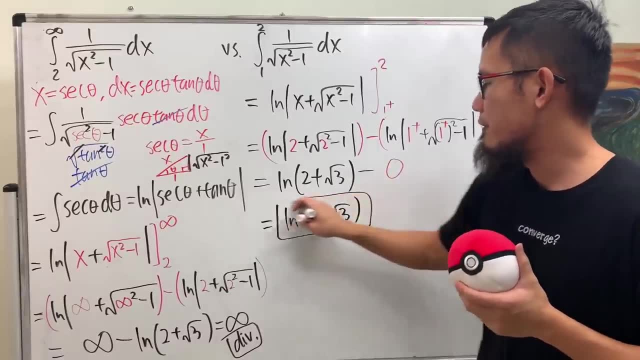 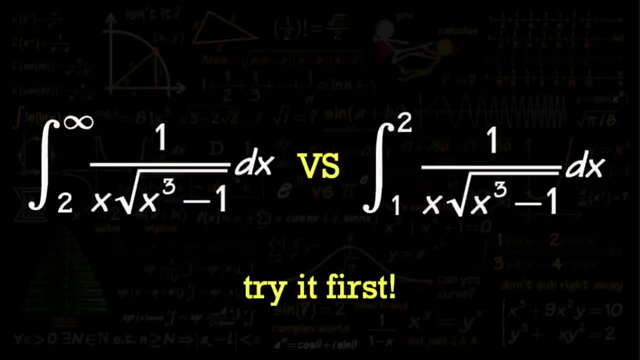 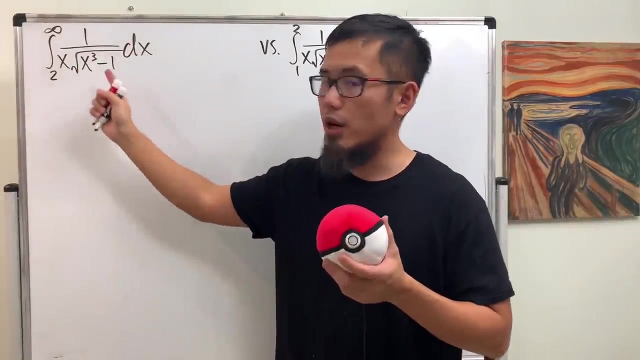 Very nice, huh. So finally, this right here converges, And it converges to ln of 2 plus square root of 3.. When we have a finite number, that will be your answer. Yeah, To integrate 1 over x, square root of x to the third power minus 1.. 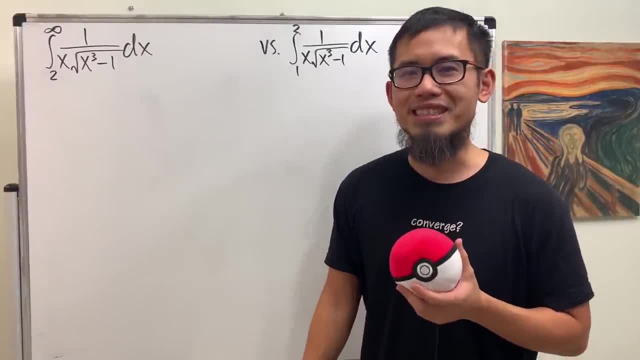 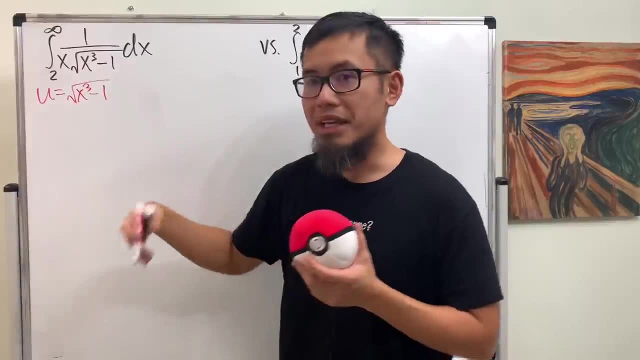 You know I like to ask these kind of questions. Don't do tricks up. You size it enough, So have a look. I'm going to let u. equal to the square root part. Square root of x, to the third power minus 1.. 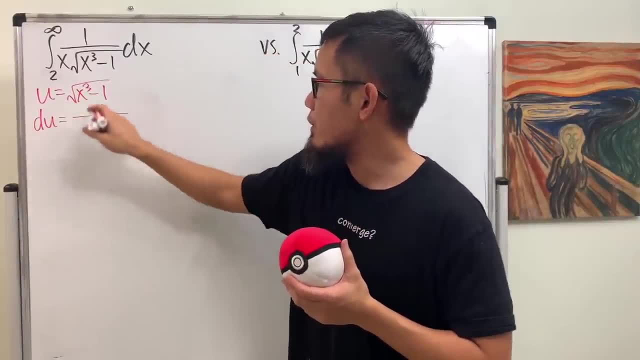 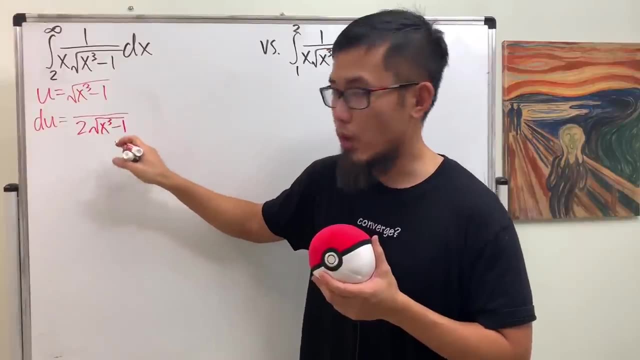 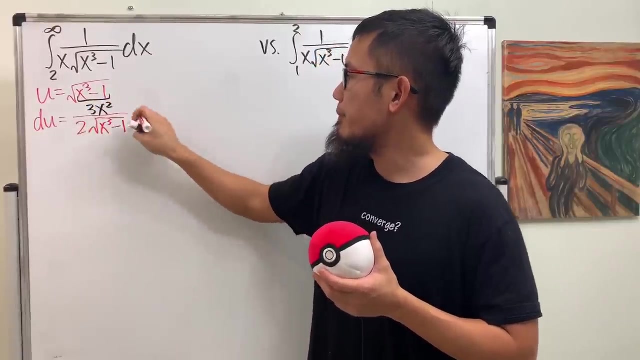 And then differentiate this, We get du equals. Well, We get the derivative of the square root over two square root. and then we have x plus third power minus one- but don't forget the chain loop multiplied by the derivative of this. so we get 3x squared right here and we still have 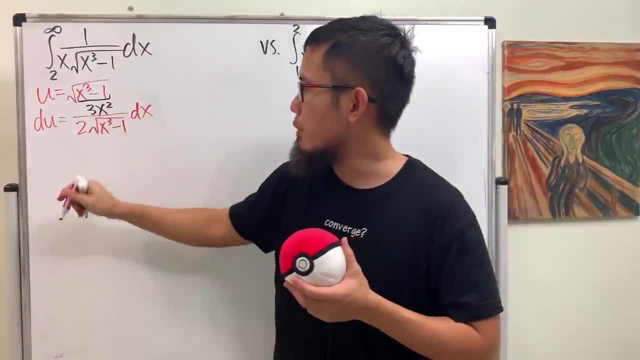 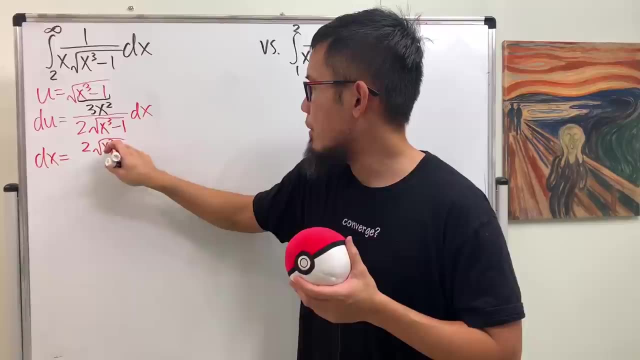 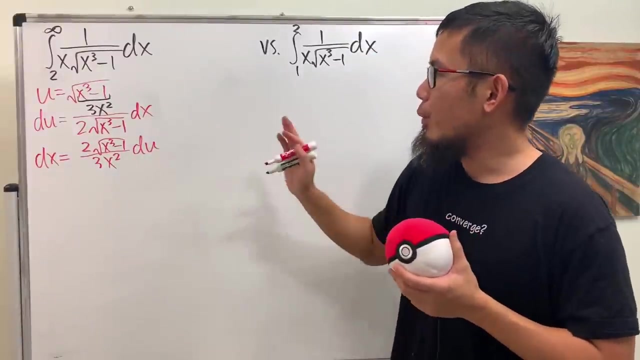 the dx, and then we are going to multiply by its reciprocal on both sides, so we get dx by itself and that's equal to two, and we have the square root of x to the third power, minus one over 3x square and we have the d u like. so now we actually have a really good choice in between of. 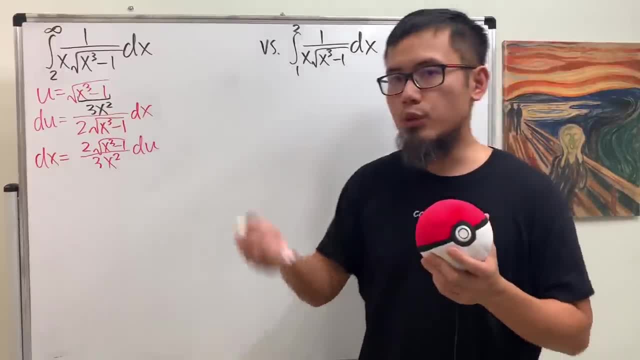 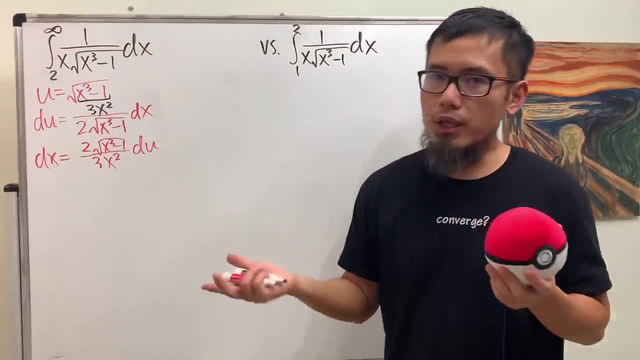 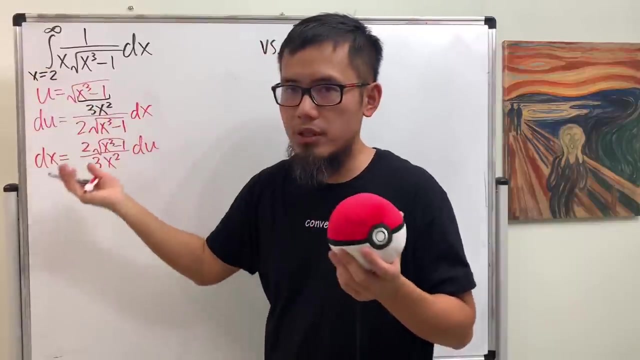 finish everything in the? u world or just do the integration first in the? u world and then go back to x and then take care of the limit up to you. in this case, i think it's okay to finish everything in the? u world because when x is equal to 2, we can plug into here, we can figure out what u is. 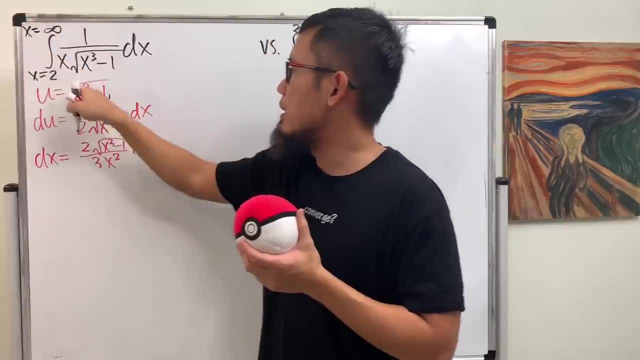 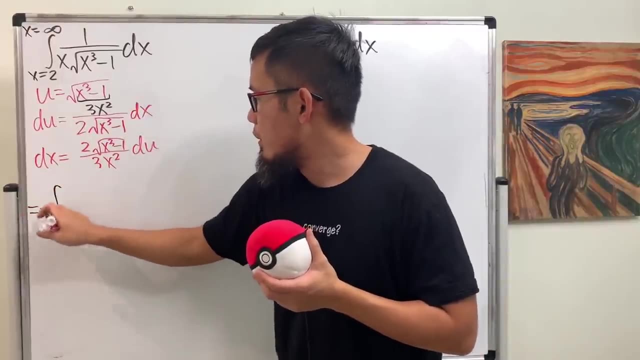 easily. and when x is infinity, again plug in here. we know what u should be be pretty easy, So let's finish everything in the? u world. In that case we will have to change the limit of integrations. When x is 2, plug in here. 2 to the third power. 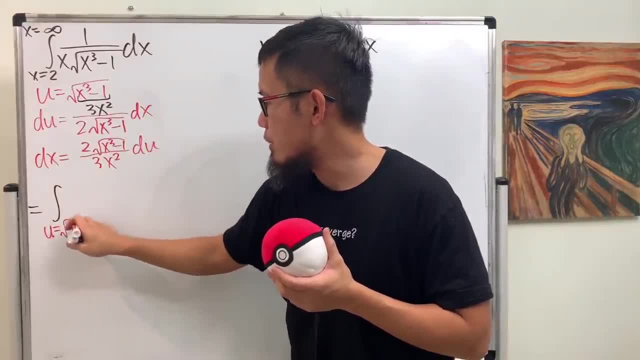 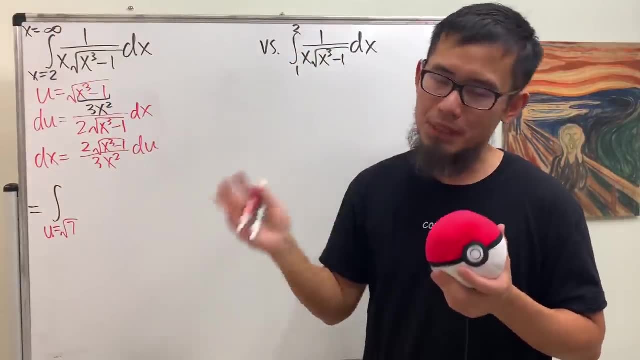 minus 1 is 7, and then take the square root, so we have square root of 7, and then we are going to put infinity to here, to the third power minus 1, and the square root of that it's still infinity. So u is still going to be infinity. Alright, now we have what: 1. 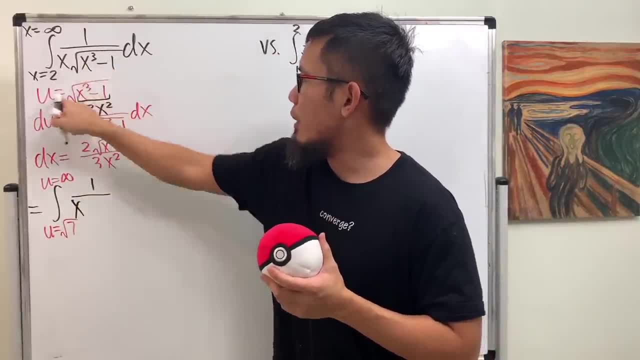 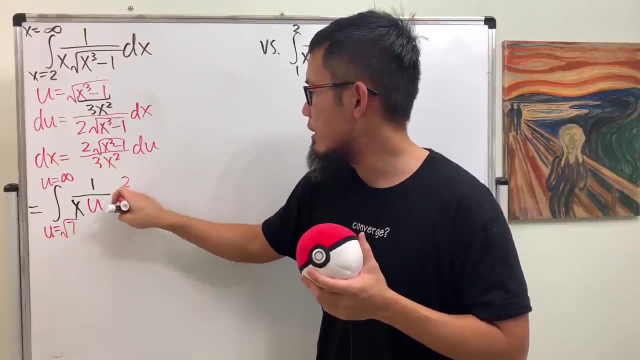 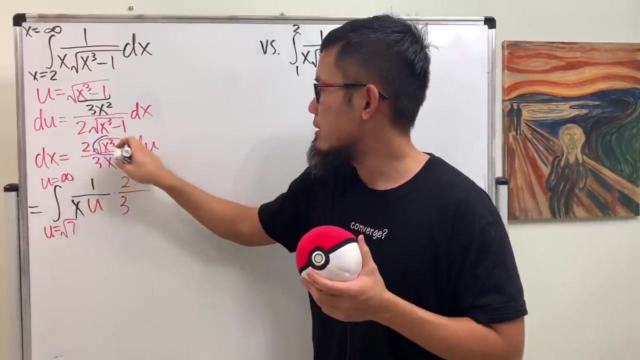 over this x, and this is our u. and then now dx is this portion. so we are going to multiply by 2, third, right, 2, third, and this guy- have a look, This is square root of x to the third power minus 1, and in fact that's our u. so we can actually just put. 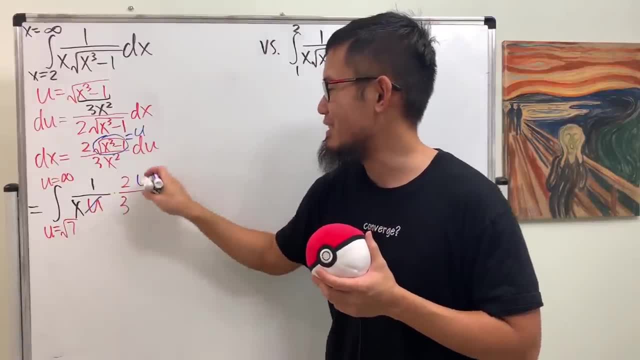 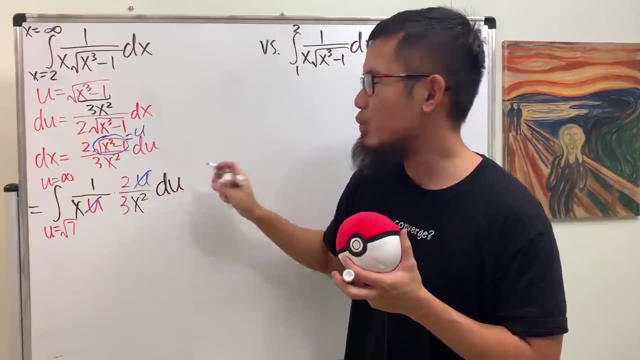 down u right here. Why do we want to do that? Because they cancel out. And then the problem here, though, is that we are going to have to take the square root of x to the third power minus 1, and we still have the x squared right here in the? u world, And you know x. 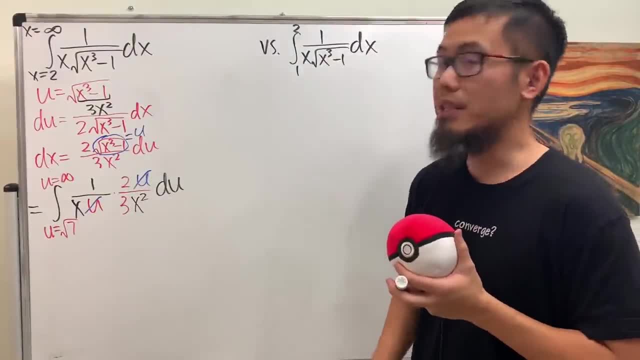 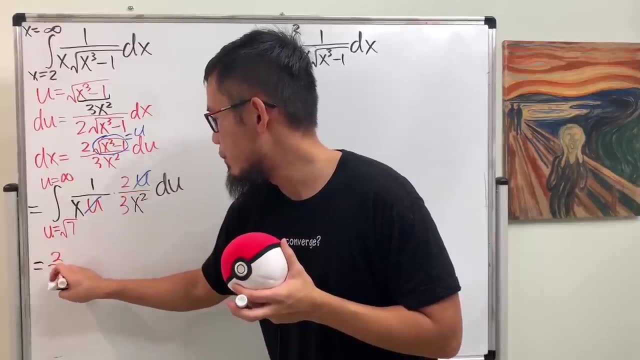 is not invited in the? u world. But it's okay, it's an easy fix. We can change it really easily. Let me write down the 2 third all the way in the front first. So here we have 2 third and we have the integral going from square root of 7, and I'm just emphasizing. 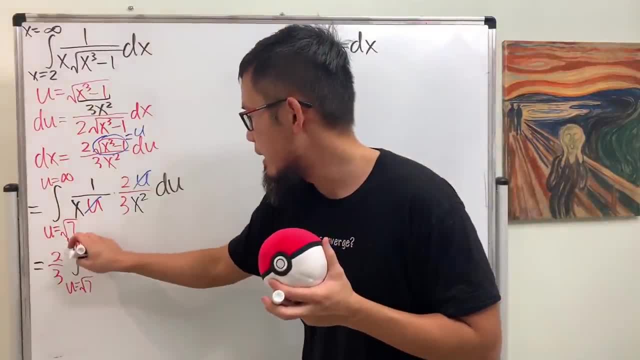 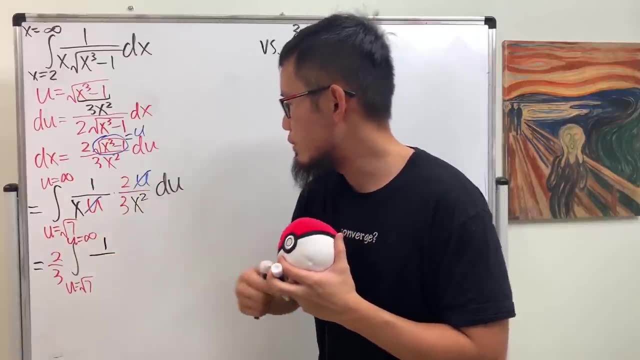 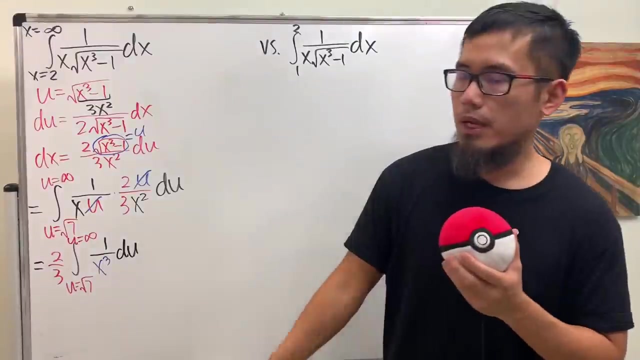 that we will finish everything in the? u world. and then we have u to infinity, that u is equal to infinity And we have 1 over x to the third power in the? u world. right, And to really take care of this business we will have to just go back here. Notice, we can square both sides. 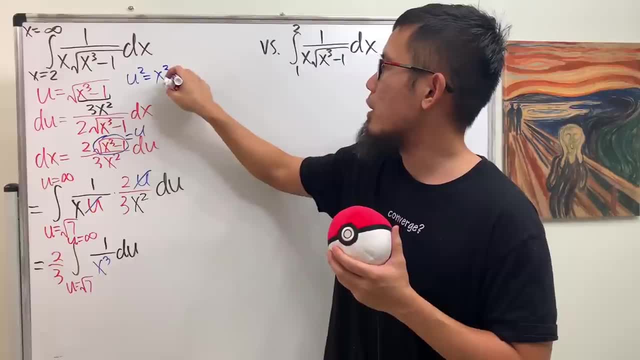 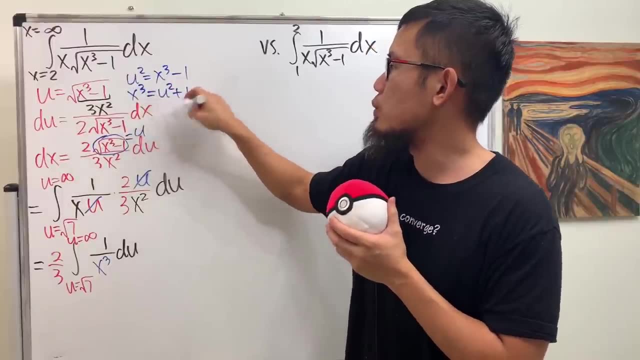 and in that case we get u squared equals x to the third power minus 1, and then add one on both sides so we can see x to the third power will be u squared plus 1.. So we can actually put this right here. 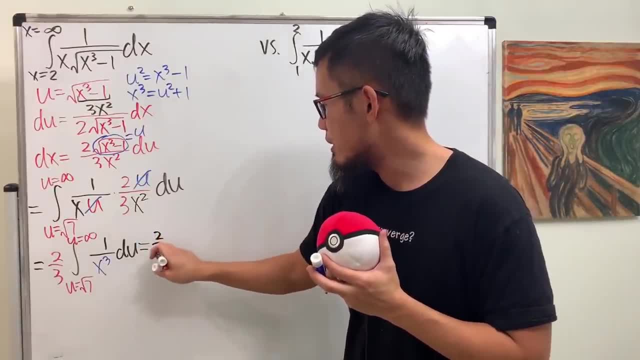 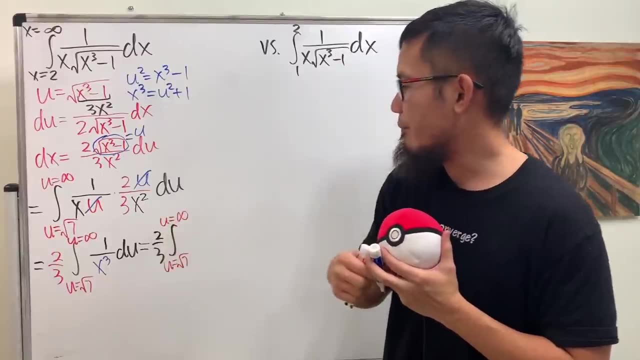 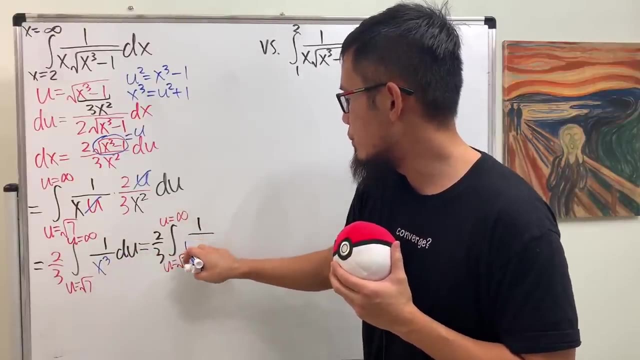 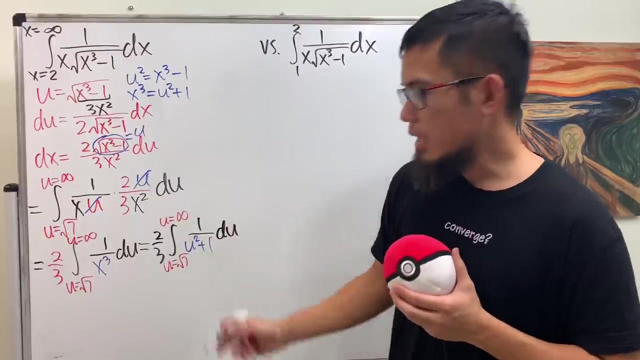 And we can integrate that. So here is 2, third integral, and we are going from square root of 7 and to infinity, like that. So here we will have 1 over the x to the third power is just u squared plus 1, and then du. Not so bad. So now have a look. Here we get 2. 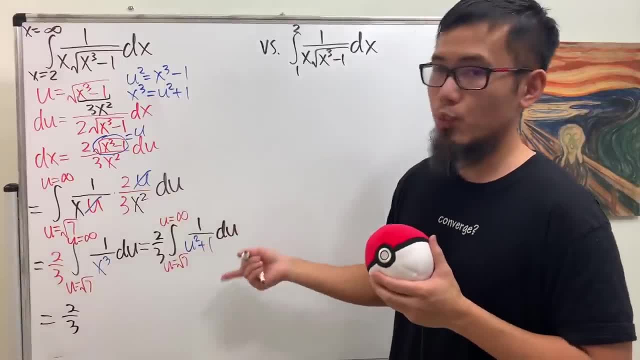 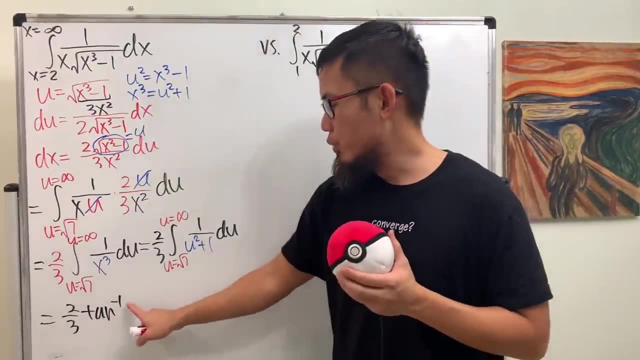 third, and 1 over u squared plus 1.. So here we have 1 over x to the third power is just u squared plus 1. in the? u world gives us precisely inverse tangent. And the best part is that if you put down u right and if you change the numbers right here, already you 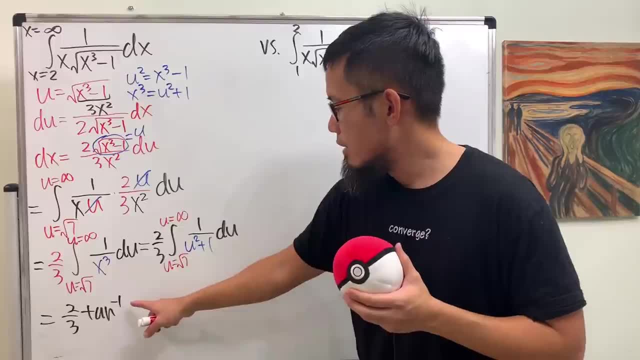 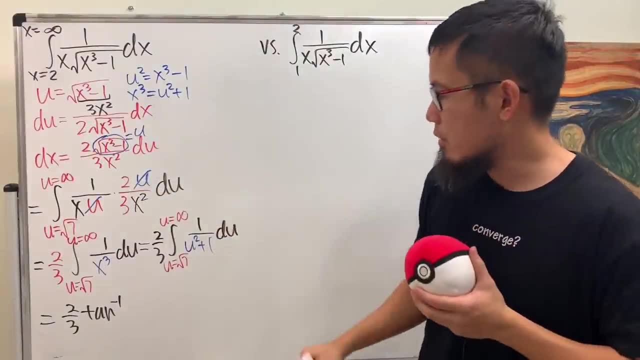 can just plug in these numbers. If you haven't put down the, if you haven't changed the numbers right here, you put down u. well, you just have to put down this expression, and you will still end up with the same thing. Anyway, though, so we have inverse tangent of u right. 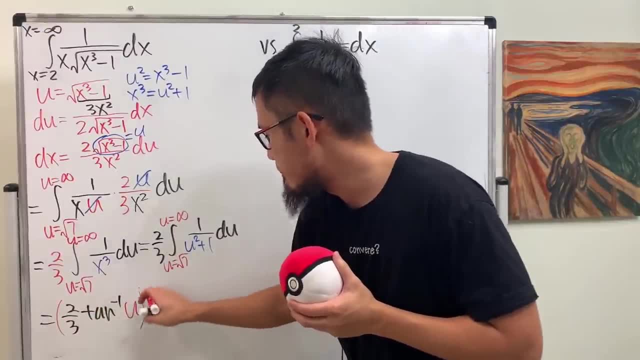 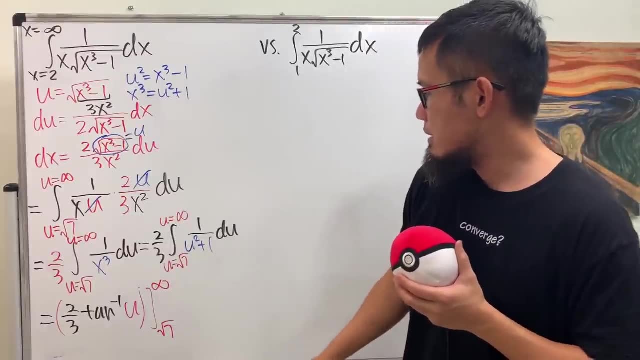 here, and then we are just going to be plugging the numbers. So here we have square root of 7, and then infinity, right? So let's see, I might not have enough space. I'll just keep writing down like this, right? So here we have 2. 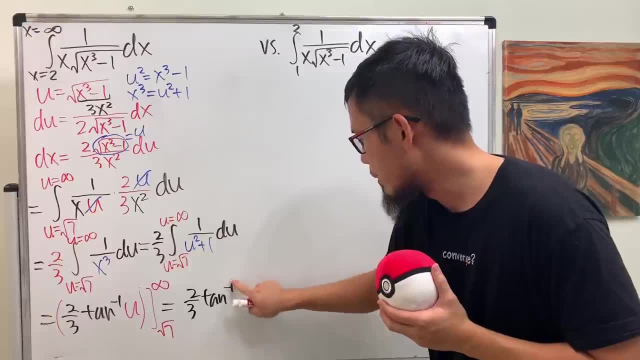 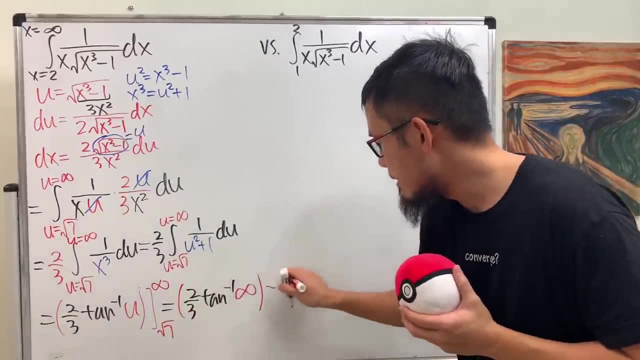 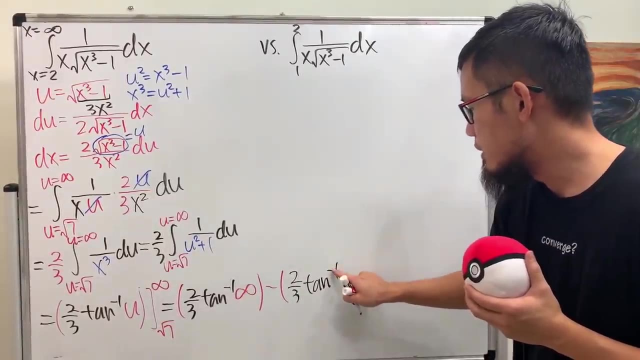 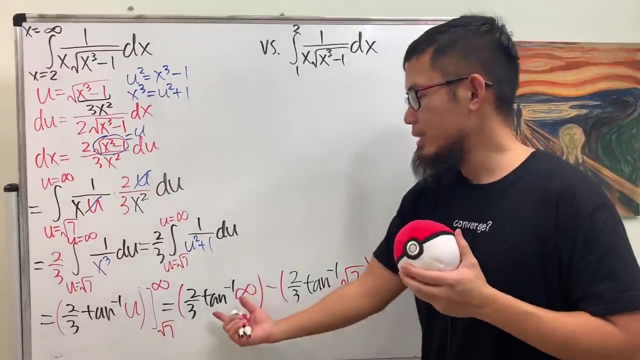 third inverse tangent. We put infinity right here And remember we are taking the limit right And then minus the second part, putting square root of 7.. So this is 2, third inverse tangent of 7, like: so All right, Now, here is the deal. What's inverse tangent of infinity? 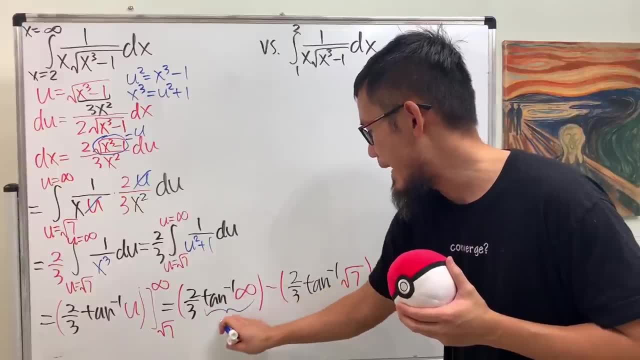 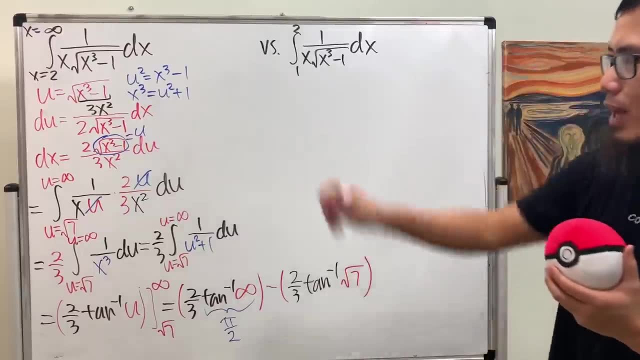 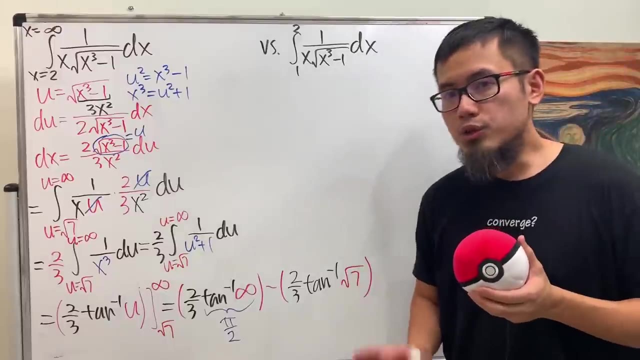 This right here approaches pi over 2, right, So that's actually very nice. This is finite. That integral actually converges. But you might be wondering what's inverse tangent of square root of 7?? You just have to know some nice angles, such as inverse tangent. 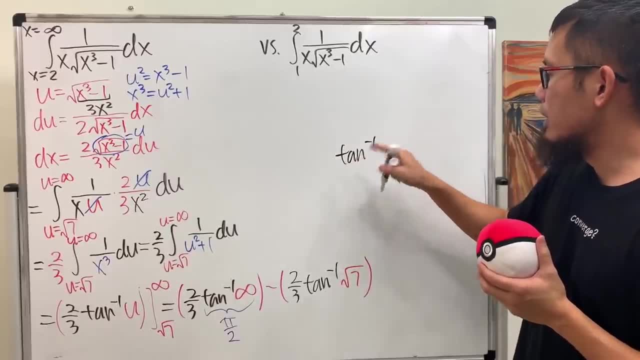 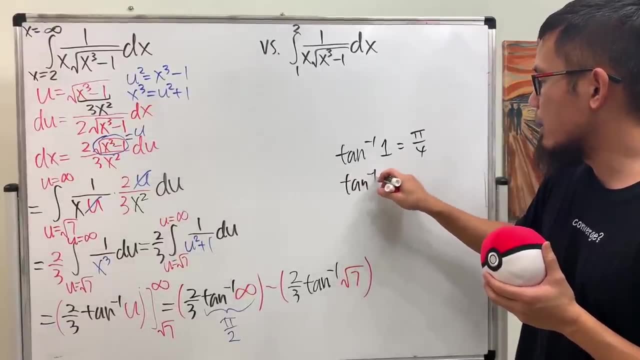 of 1.. Like, for example, you just have to know the inverse tangent of 1 is pi over 4.. And this is a really common one. And then I'm also going to ask you guys to try to figure out the inverse tangent of square root of 3.. I think you guys can also figure this out as 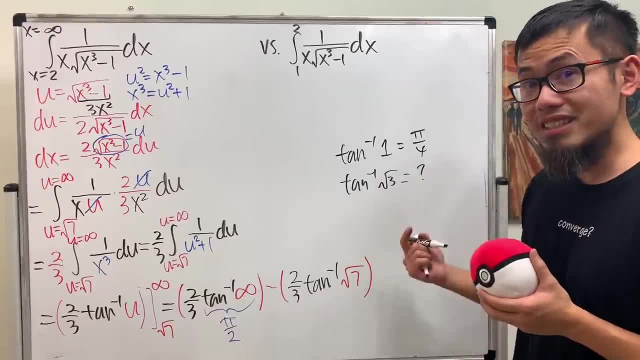 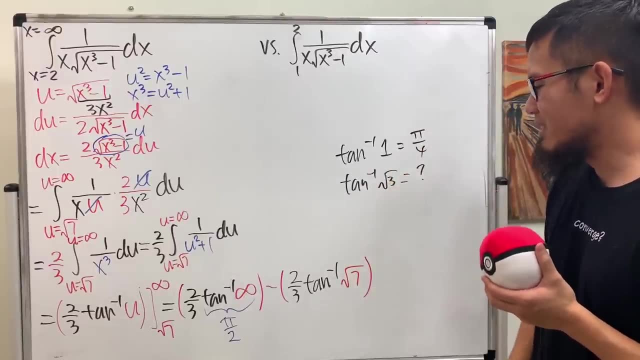 well, Think about it. Leave a comment down below. Is this pi over 6 or pi over 3?? Notice that these right here are just special angles. But when you have square root of 7 like this, eh, we'll just leave it like that. That would be totally okay if you do that on my exam. 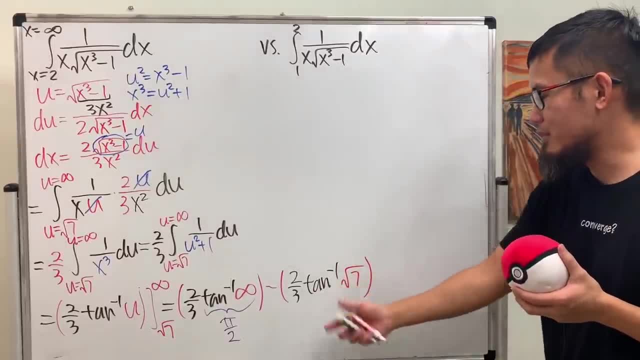 Unless this is all right, then I'll just leave it like that. And then I'll just leave it just like that. There's also a special angle. You can tell me the angle of this right here? The term is thought to be like 13.75 degrees. I don't know, though. I just made that up. 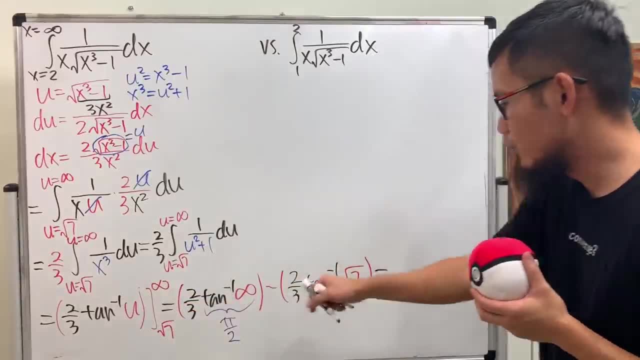 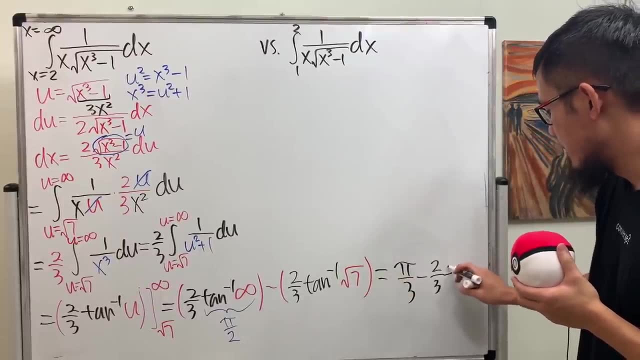 Anyway, though, 2 third times pi over 2, the two cancels, So we have pi over 3.. So that's very nice. And then minus this is still a finite number. So 2 over 3, inverse tangent. 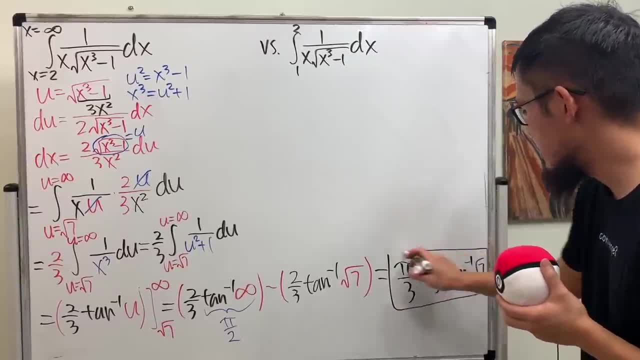 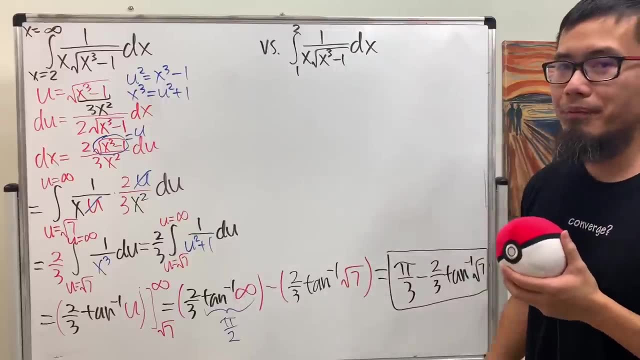 of square root of 7.. So this right here is the first one, So it actually converges Very nice. Now have a look right here: When x is 1, we get vertical asymptote right, Because we will produce a 0 in here. 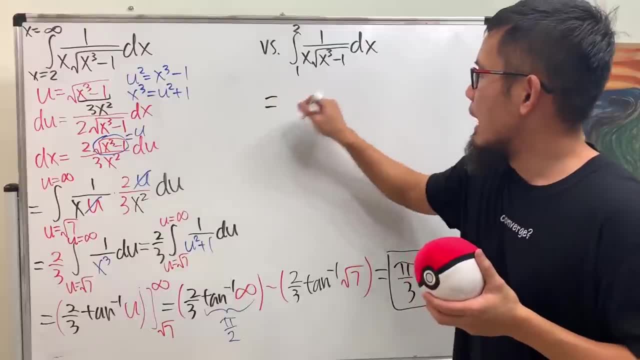 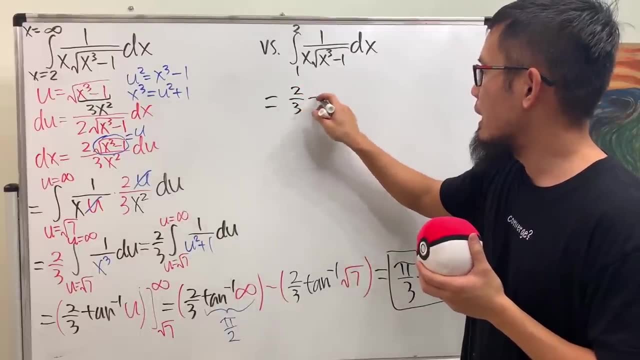 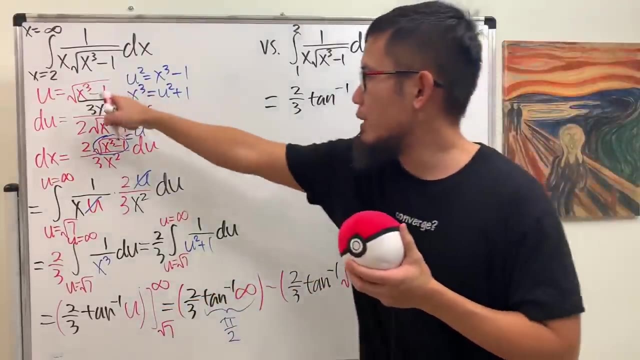 All right, fine, All right. I'm just going to pick it up from here, because it's going to be the same integral. So this is going to be 2, 3rd and we have the inverse tangent right. And now here I use u and u was equal to that. 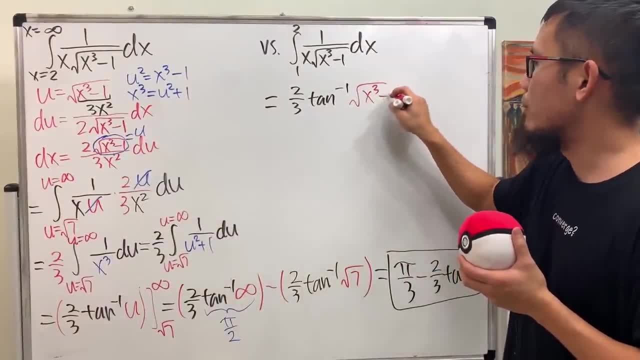 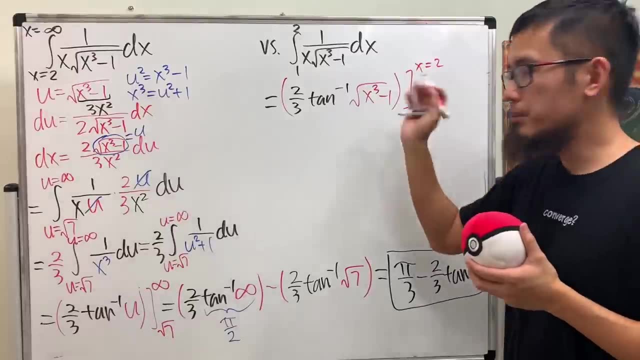 so I'm just going to put in square root of x to the 3rd power minus 1.. Right, And of course in this case we are talking about when x is equal to 1 to 2.. Plug-in, plug-in, and technically this is 1+. 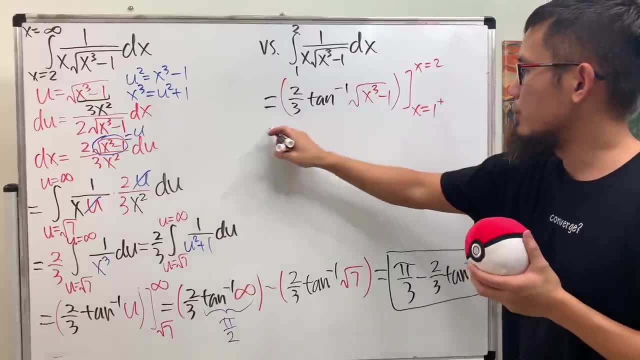 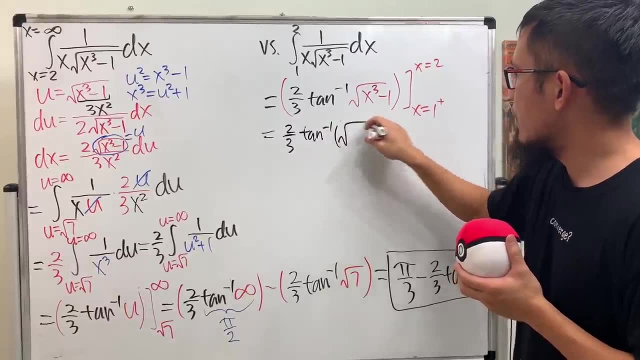 but it doesn't really matter that much. Anyway, plug-in 2, let's see what we get. This is 2, 3rd inverse tangent of square root of 2 to the 3rd power minus 1, and technically it should put a little parentheses. 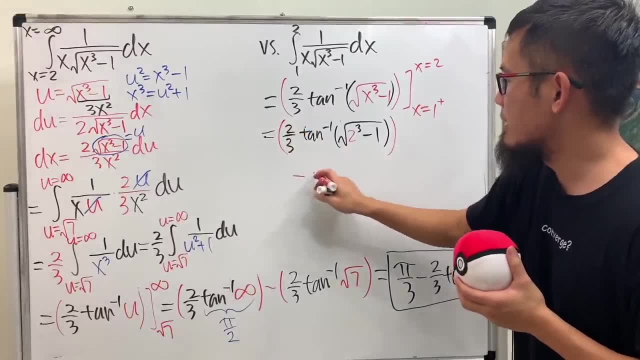 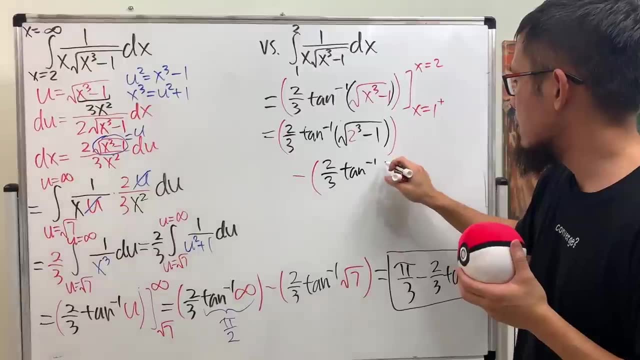 All right. so that's the first part, and then we have to minus the second part. It's putting 1 plus in here, So 2 3rd inverse tangent of square root of 1 plus to the 3rd power. 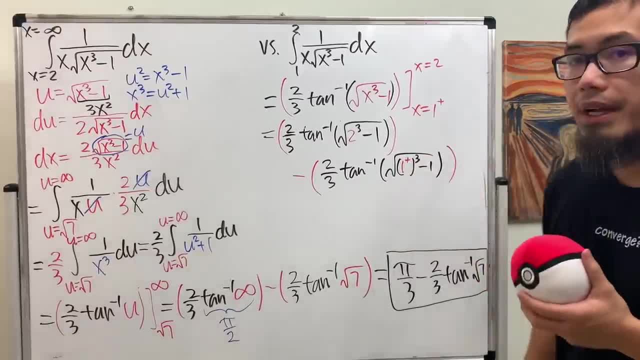 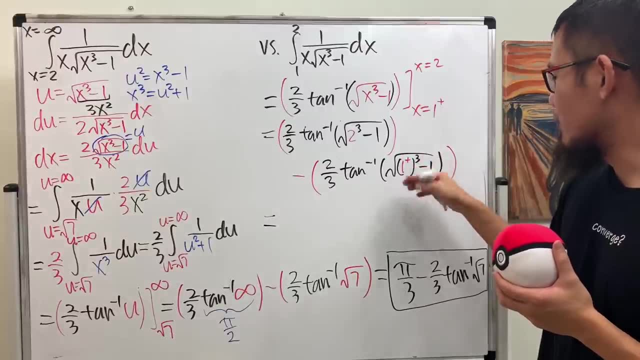 and then minus 1, like: so All right, This right here is what: 1 plus 3rd power, or 1 plus plus 3rd power is still 1 anyway. Minus 1 is 0, so this thing is actually just 0,. 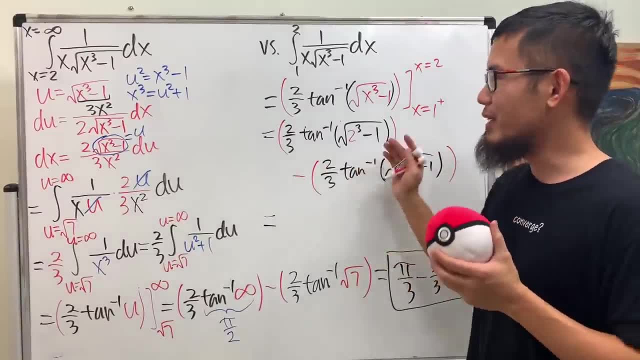 so this thing is bye-bye right. So that's actually very nice. This right here is 1 plus 3rd power, and this right here converges as well, because whenever you have the triple place, that gives you a finite result. 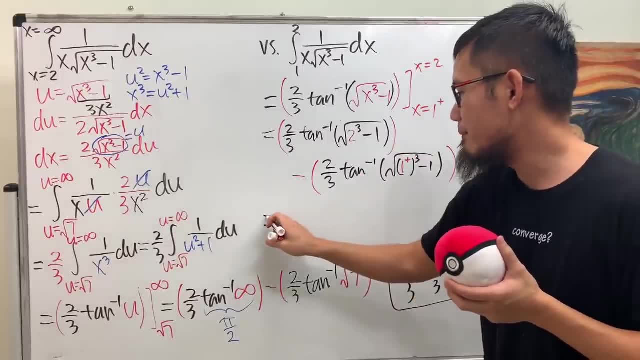 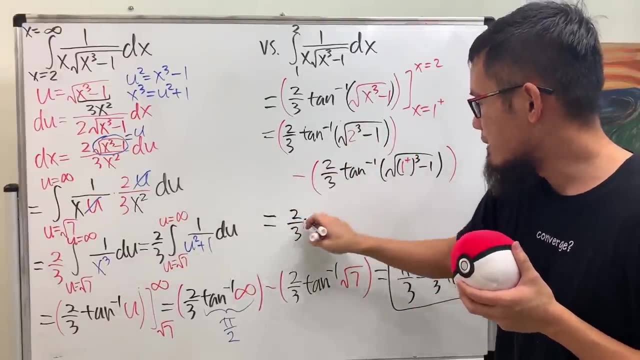 like 0 or whatever you know. the rest will be fine, And for this it's just that right. It's just going to be square root of 7.. So this is 2 over 3, inverse tangent of square root of 7.. 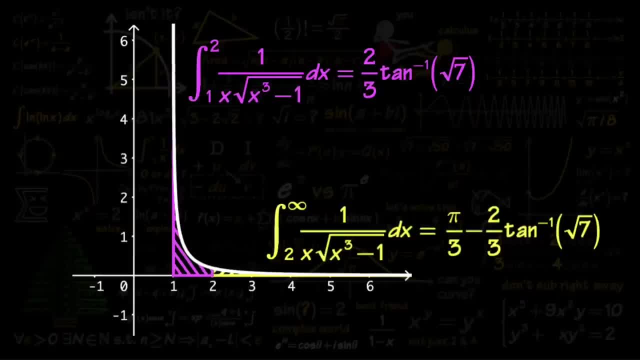 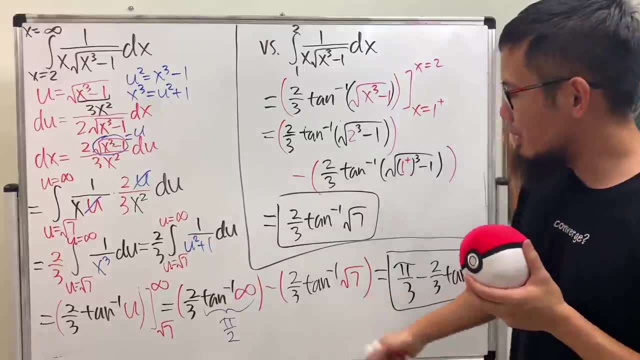 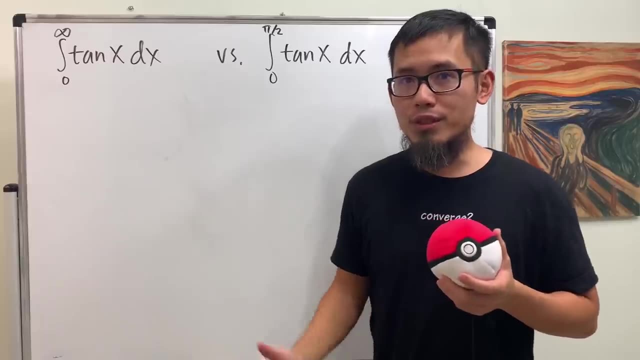 Yeah, So very cool, huh? In this case, when we have the type 1 or the type 2 situation, they both converge. They both converge. Check that out First. we know the standard result for the integral of tangent x. 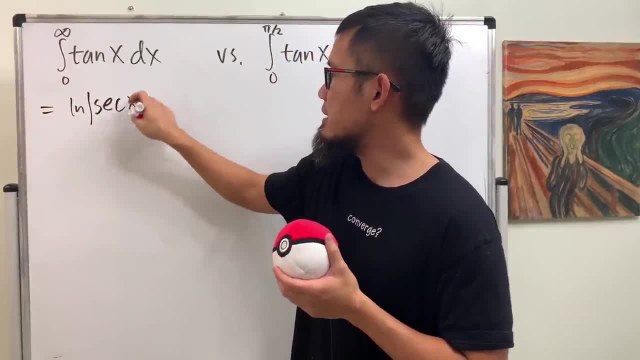 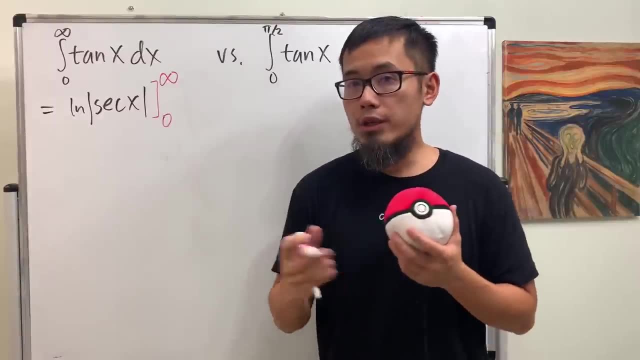 which is just ln, absolute value of secant x. And now we are going to go from 0 to infinity. But remember, when we put infinity into the function, we are talking about the limit, right? So pay attention to this one. 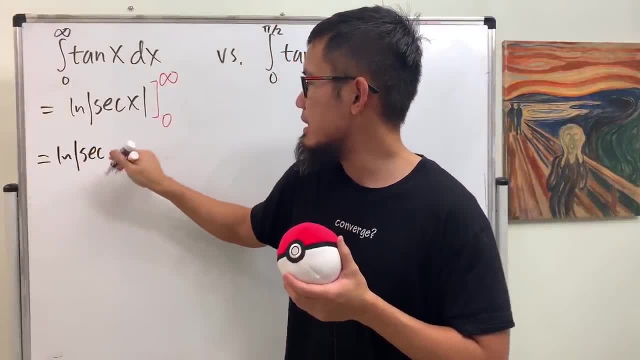 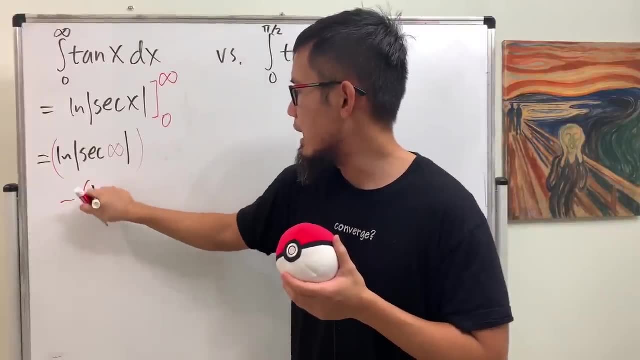 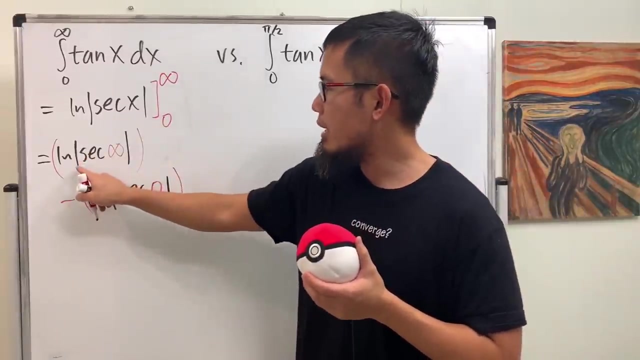 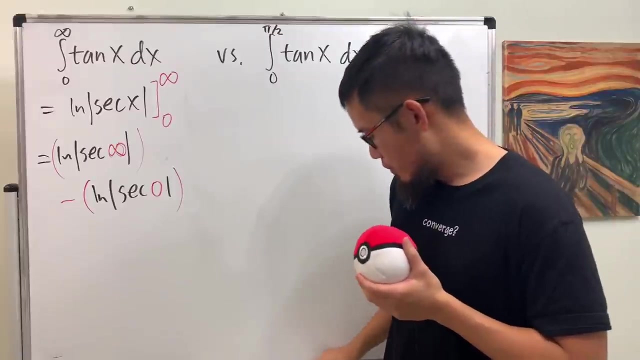 If we just write it down as ln- absolute value of secant infinity, and then, because that's the first part, let's put parentheses around it and then, minus parentheses, ln of the value of secant zero. well, what is ln of what's secant of infinity? how do we do this one? hmm well, whenever you are in doubt, in terms like about: 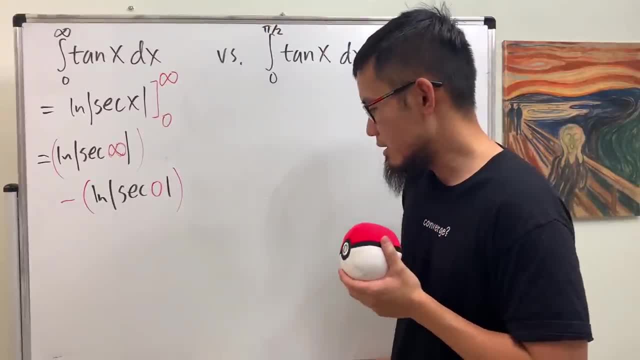 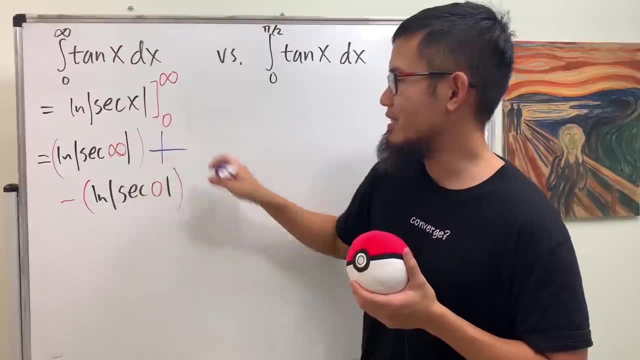 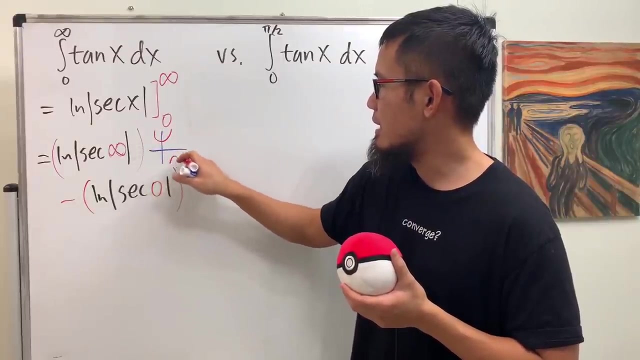 uh, limits or whatever. the best thing, one of the best thing, is to look at its graph. so let's go ahead and just, you know, look at the graph. so let me just remind you guys. maybe you haven't seen this for a while. the graph for secant x is like this, like it's like this and then like that it. 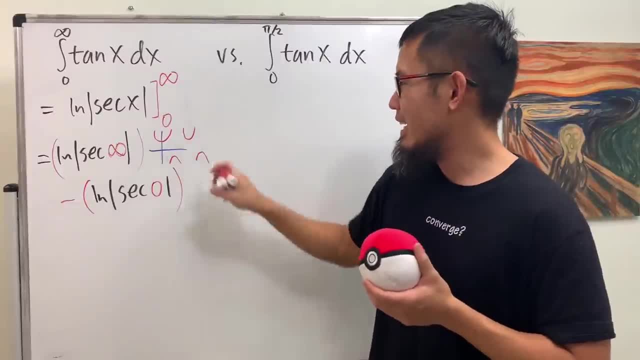 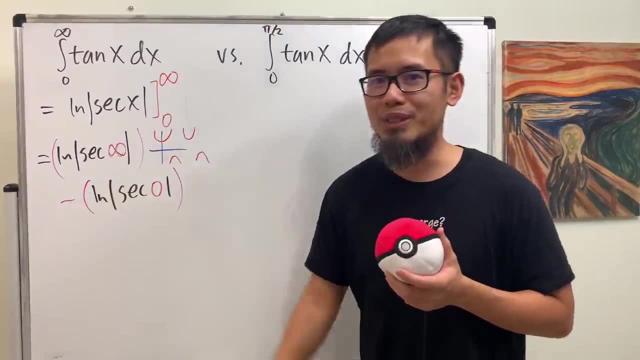 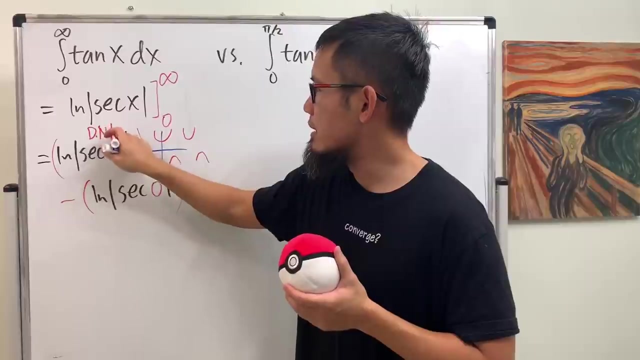 has a lot of the u's right. it has a lot more, of course, and when x is approaching infinity, this right here is behaving really, really wildly. in another word, there's actually no limit for that. so this right here, it's not infinity, though is does not exist. 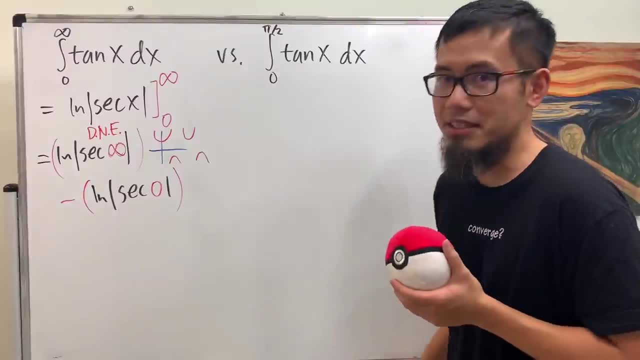 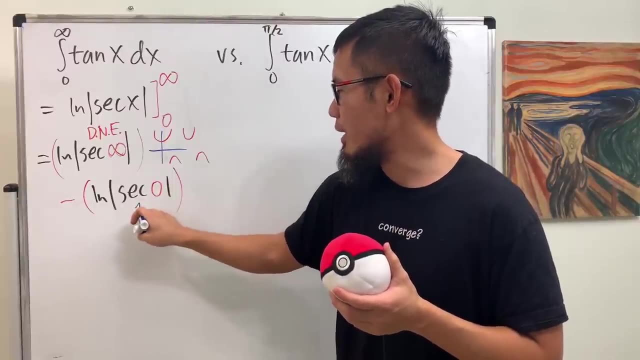 and, of course, when you have ln of does not exist, that just does not exist. but, by the way, i just want to give an honorable mention: secant of zero is equal to one, but that doesn't matter if you have does not exist plus or minus or whatsoever. 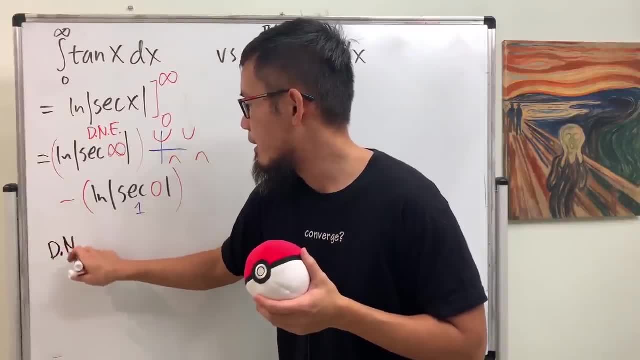 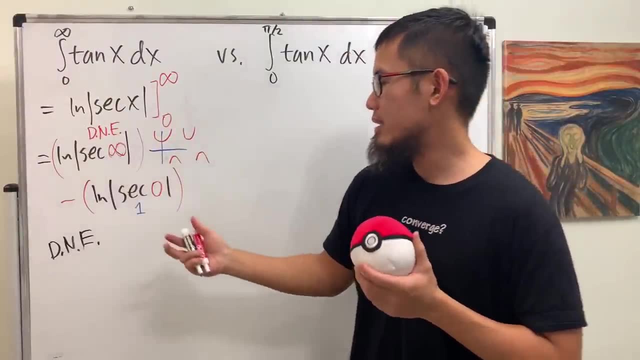 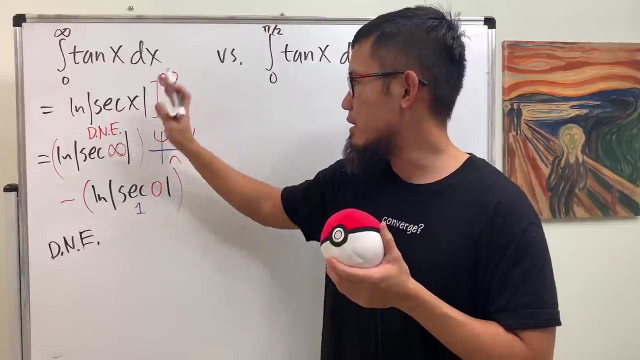 this right here just doesn't exist. because, keep in mind, whenever we are doing an improper integral, we have to take the limit and the limit. we might get a situation that does not exist, but you don't have to be saying anything crazy because as long as you don't end up with a finite value for the improper integral, you can just say: 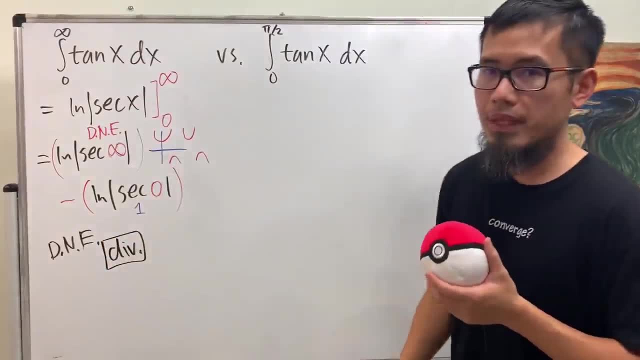 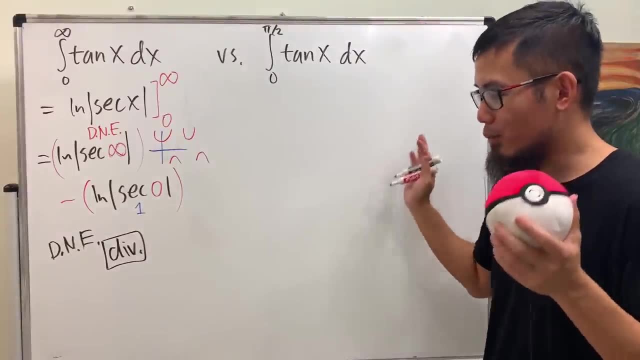 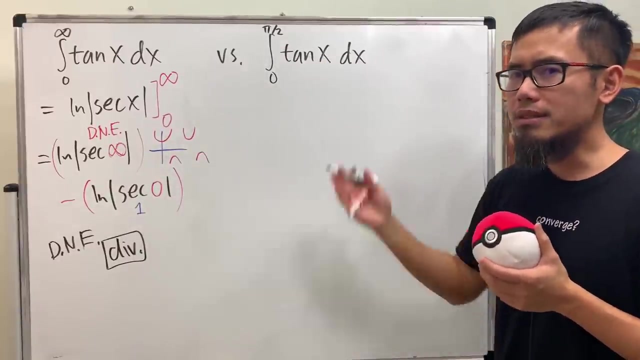 this integral right here diverges, but you cannot say it diverges to infinity anymore, right? you cannot say that. you can just say it diverges and walk away. that's all now. have a look right here. this time we have from zero to pi over two. why is this improper, though? 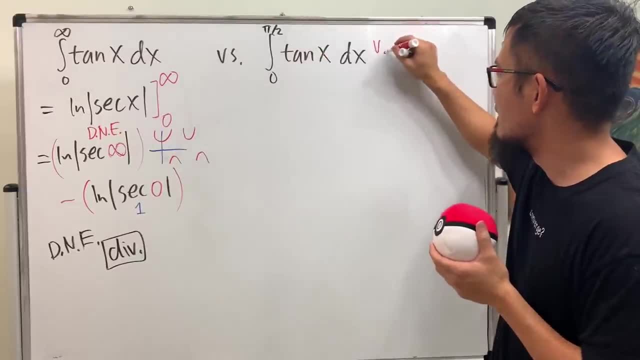 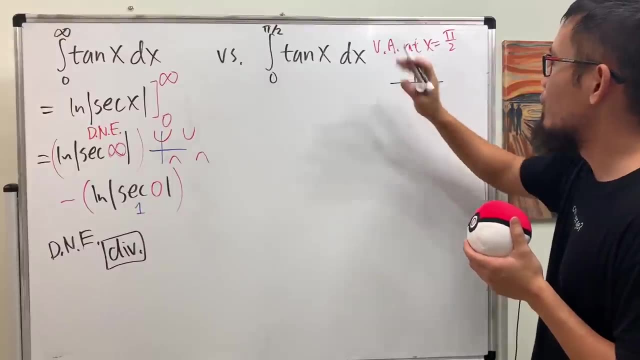 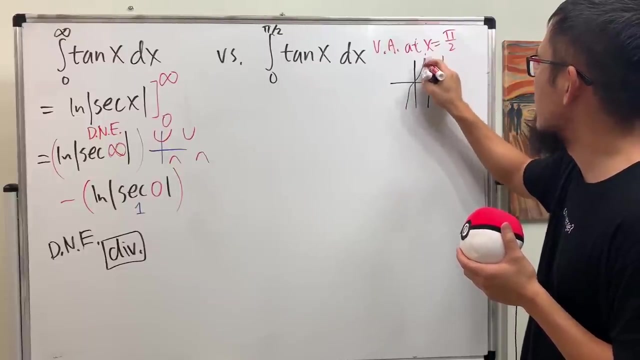 okay, yes, we have a vertical asymptote at pi over two. very nice, right? so, just as a reminder, when we have the graph of tangent, it looks like this, right? so it's bunch of these guys. and when x is pi over two, it's right there. so we have a vertical. 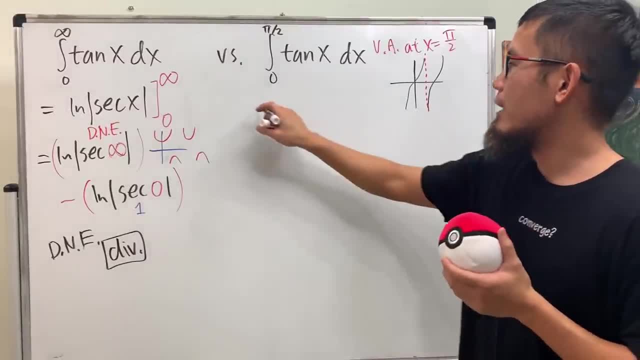 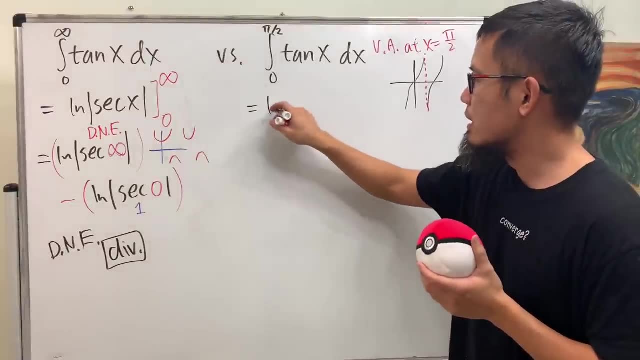 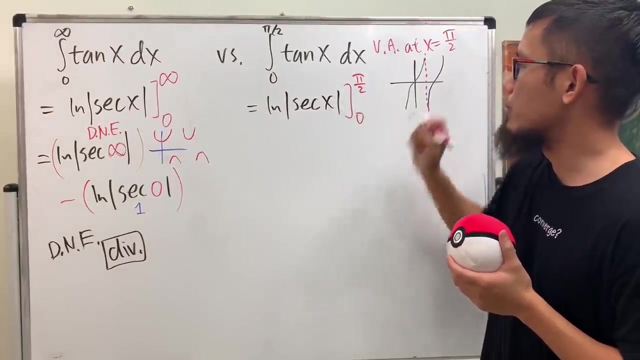 asymptote. that's why this right here is improper. I always mention the vertical asymptote when you are dealing with the type 2 situation. for the proper integral. all right for this again, natural log of بعدs 不凡. then plug-in to x. 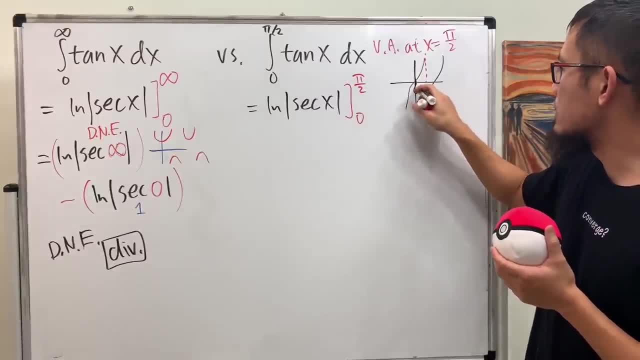 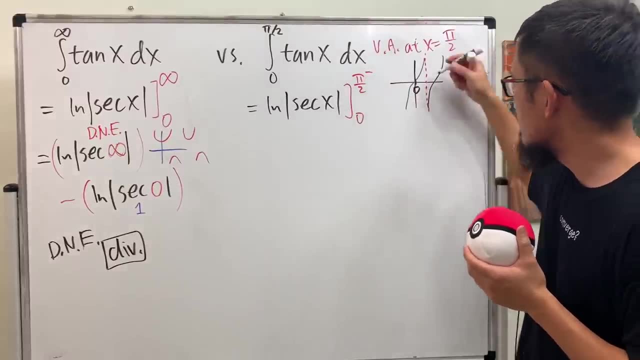 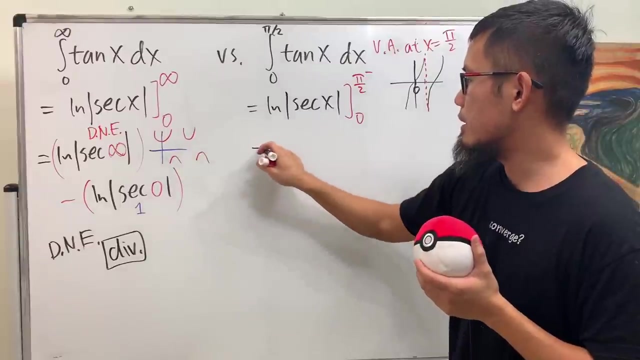 but technically though this time, because we're going from 0 to pi over 2, this is pi over 2 over 2, minus right. you are approaching pi over 2 from the left hand side, like right here. i thought that's the pi over 2. a little bit of that, all right. here we have ln absolute value of secant. 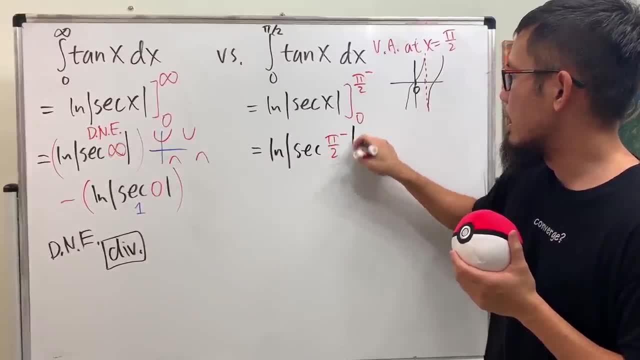 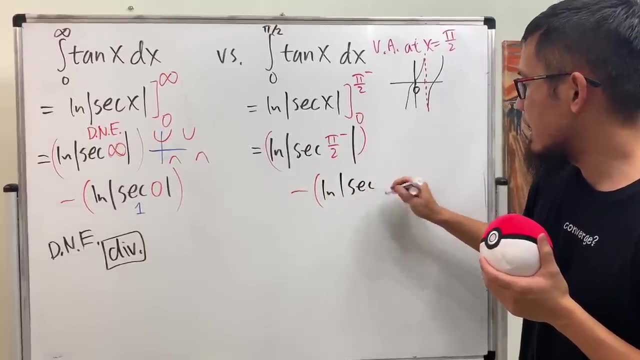 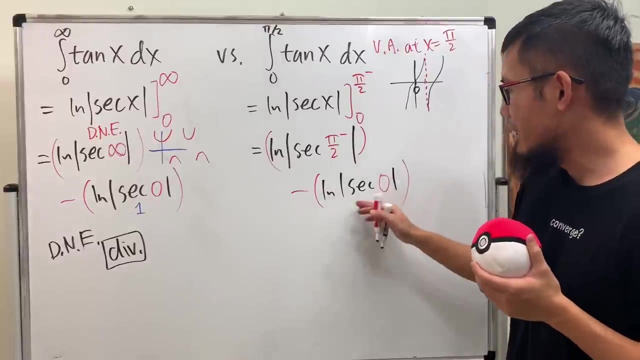 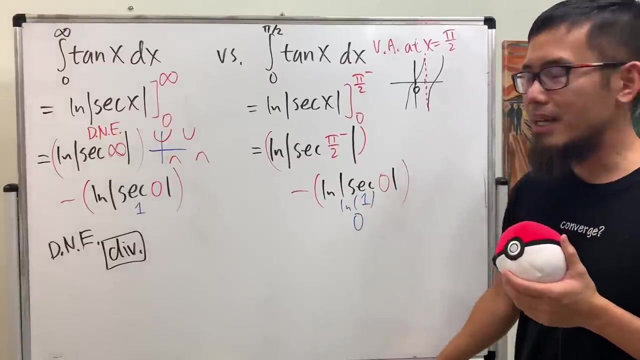 pi over 2 minus. and then that's the first part right minus the second part. ln. absolute value: secant: 0. all right, this right here is 1, ln 1 is 0, so all in all this is just 0. that's nice, but the question is, what's secant of pi over 2 from the left hand side? 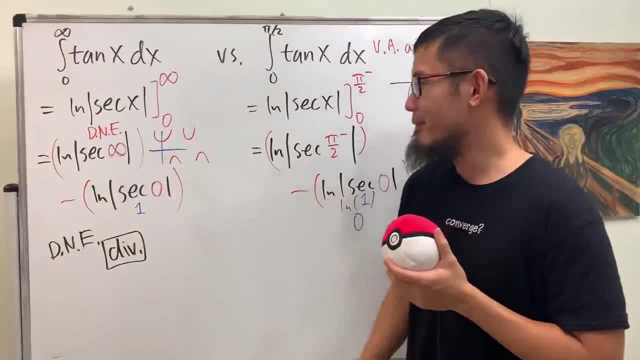 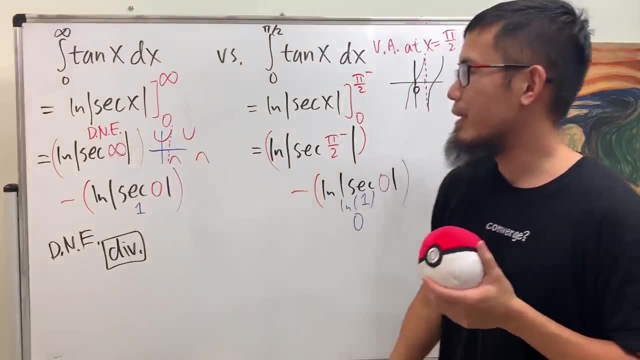 well, we're going to look at the picture again. so the the the thing between secant and tangent is that they both have vertical isotope at pi over 2 right here you, and if you go, if you go to pi over 2 from the left hand side, you see that the graph right here. 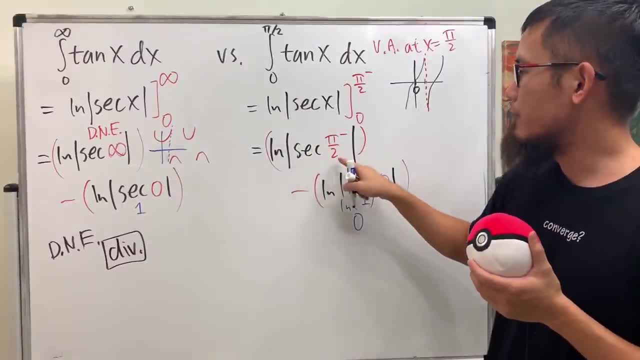 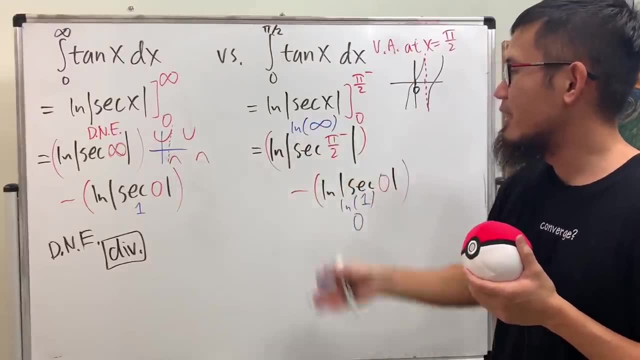 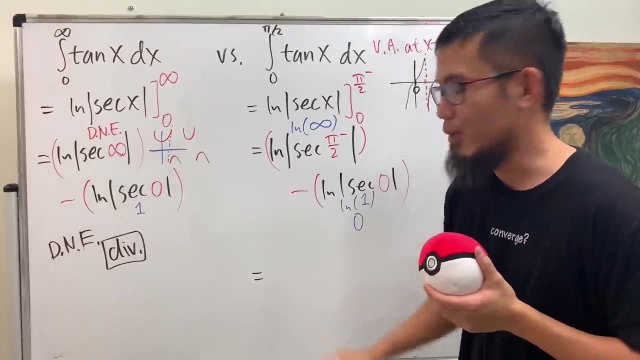 it goes straight up. so, in fact, secant of pi over 2 minus, this right here gives you infinity. and then, when you do the ln of infinity, this right here gives you infinity. infinity minus infinity: this right here gives you 0. no, just infinity minus 0 gives you infinity. so in this case,